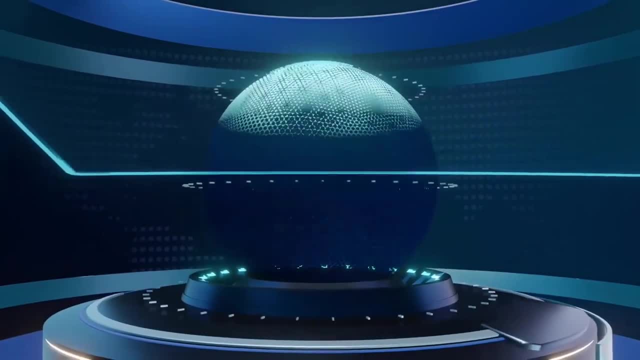 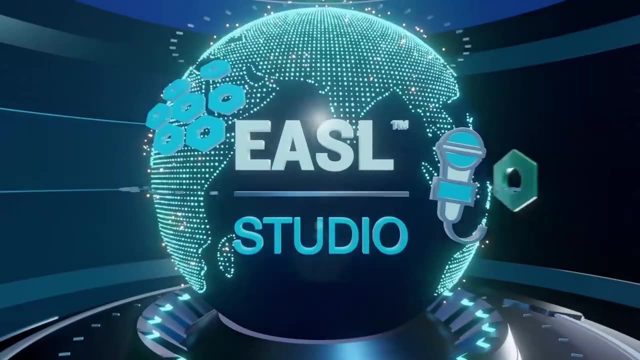 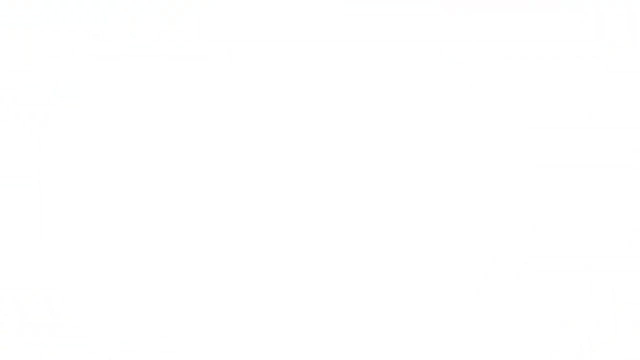 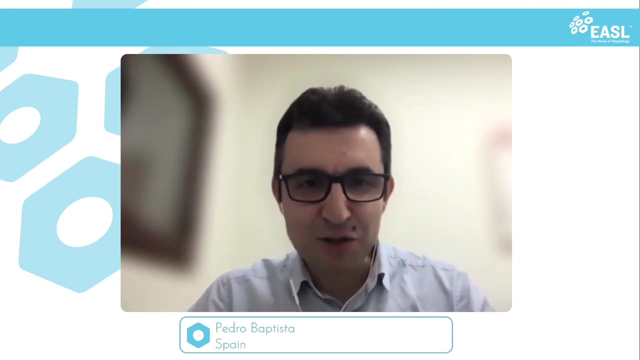 Good afternoon. It's a pleasure to have you all here and I want to welcome to the Easel Studio, your weekly hepatology broadcast news. In today's episode we will discuss regenerative hepatology, from stem cells to tissue engineering, and I actually have the pleasure to. 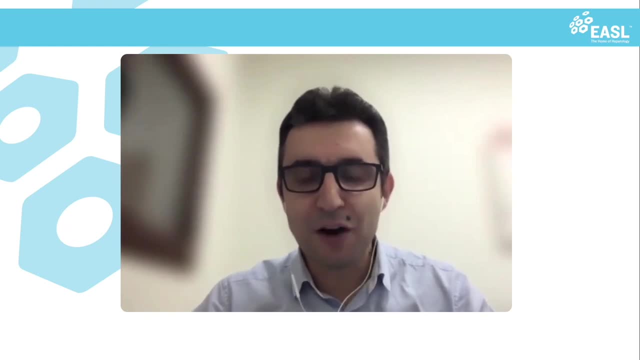 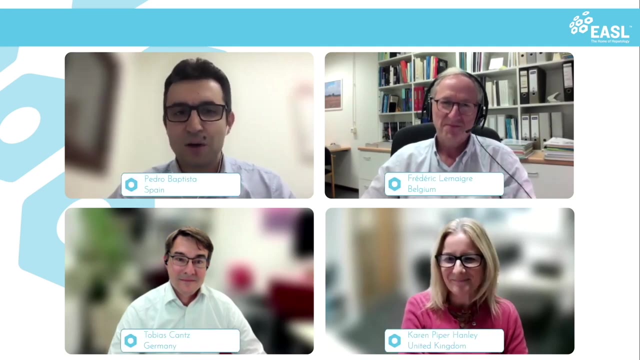 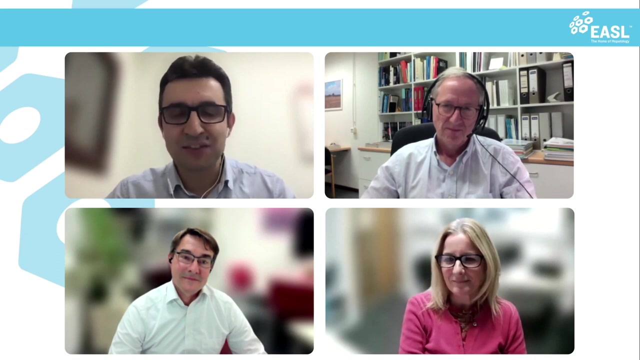 host and moderate this Easel Studio in the very good company of Professor Karen Piper Hanley, Professor Frederick Lemager and Professors Tobias Kentz. So the field of regenerative hepatology, as you all know, it is something that has been progressing in the past decade. 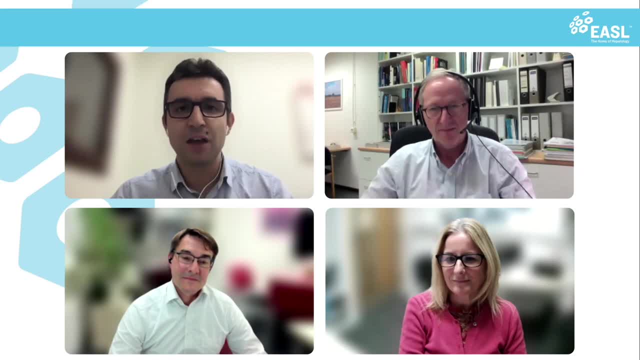 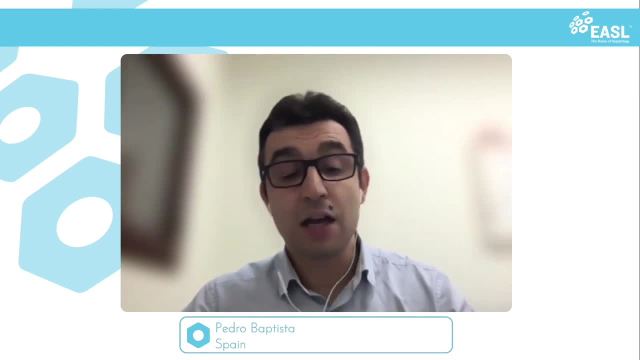 Quite fast with new therapies, with new products, trying to give answers to decades and centuries old problems, which is liver regeneration and liver disease In general. regenerative hepatology constitutes this interdisciplinary branch of biomedical research and hepatology in particular, which focuses on the developing science and tools to repair or replace the 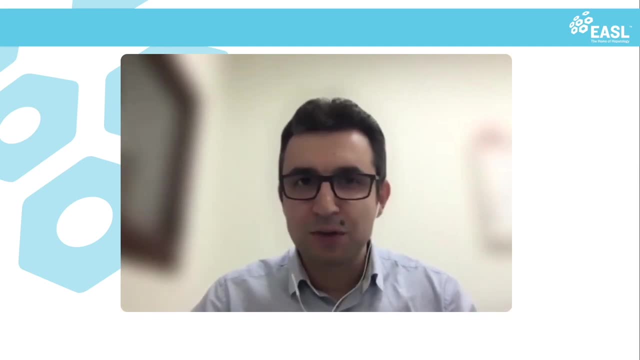 damaged liver. So you might work in liver fibrosis, liver steatosis, but in the end I mean, most of you actually are working in regenerative hepatology because, as we are, you're also trying to repair and regenerate the liver. So in the end, I think we're all pretty. 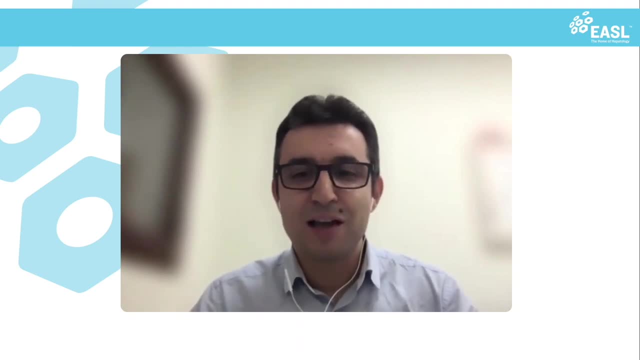 much in the same basket, or pretty much working in the same field, towards patient's good, I would say. So major contributions in this effort derive from tissue engineering, stem cell biology and addictive manufacturing, And this is actually where Easel has been, I would say, at the forefront of. 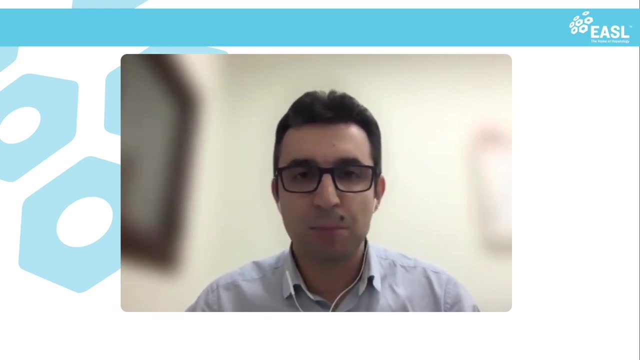 regenerative hepatology. So, for example, a few years ago, by initiative of Professor Massimo Pinzani, a group of us actually put together what we call now the Easel Consortium for regenerative hepatology, which really addresses a lot of these problems, And historically we have been devoted to. 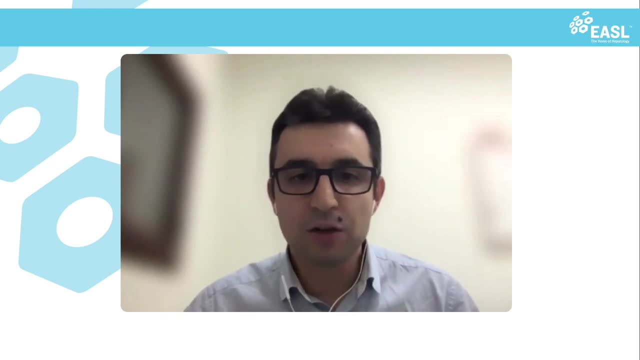 three main research programs, or three pillars as we call them, To develop cell therapies in bioengineered bile ducts to be used in liver transplants and congenital biliary diseases, create a 5-10% in order that we can treat or to implant this in treat inherited hepatic metabolic diseases. 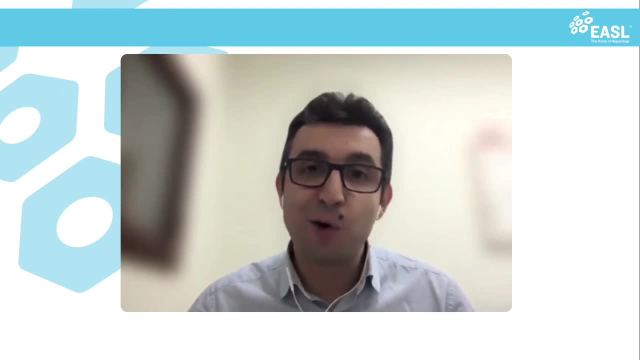 and then our ultimate goal- which i think it's actually the goal of many people here listening today and now, and worldwide- at least patients also want this- is to create more than 30 percent bioengineered liver mass that we can transplant in patients with acute, acute on chronic liver failure. 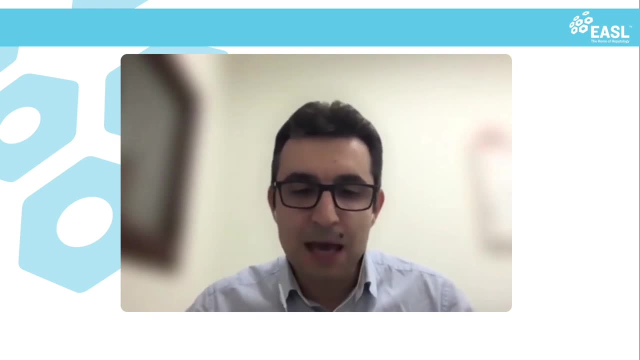 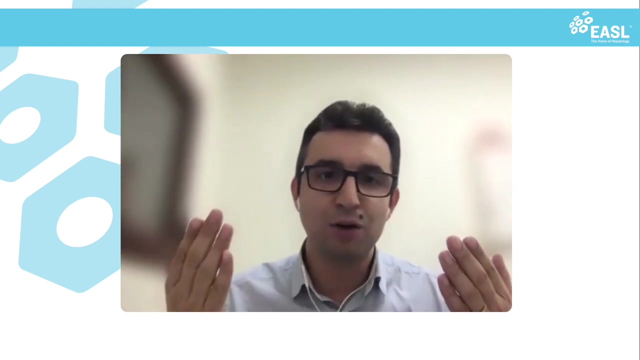 and, as you guys know, so there's very many, many challenges in this. there's many things that we still need to do, but the field is not only devoted to this, and when you look into stem cells, cell therapies, small molecules, tissue engineered products, gene therapies and then the ultimate goal, 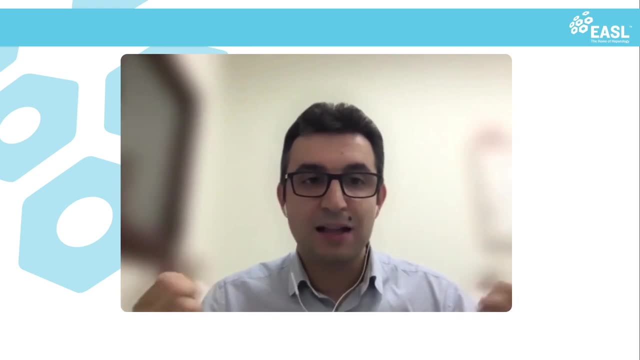 of liver bioengineering. there's really a lot that we need to do, and this is exactly what we're going to be discussing today, and we'll start with the basics. i would say we started back in the 90s with cell therapies, but where we are today, we're still, i think, a little bit far away from a validated 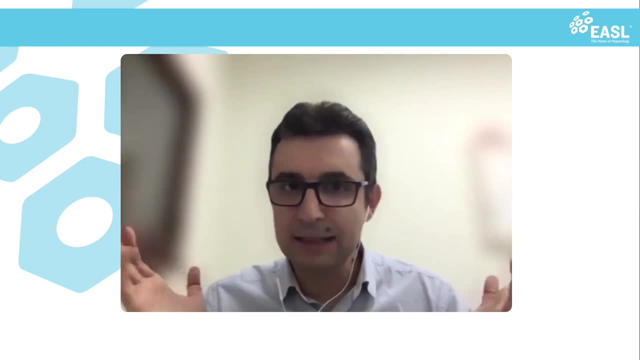 reproductive or reproducible stem cell therapy or any type of liver cell therapy that can actually heal patients in a more or less predictable way. and this is where i pass the word to to my friend, to bs khans, and ask him: so what do you think we need to do to actually make this field actually? 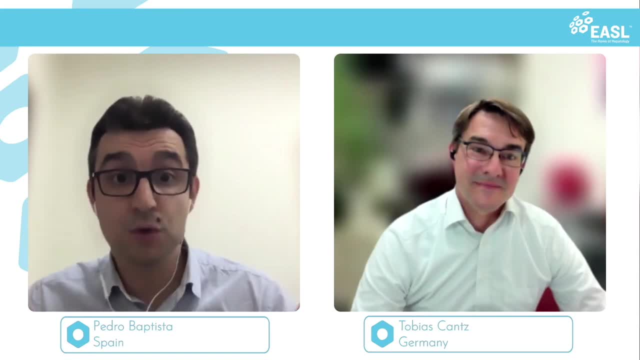 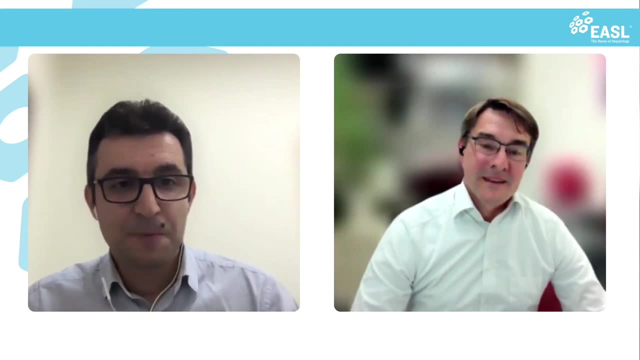 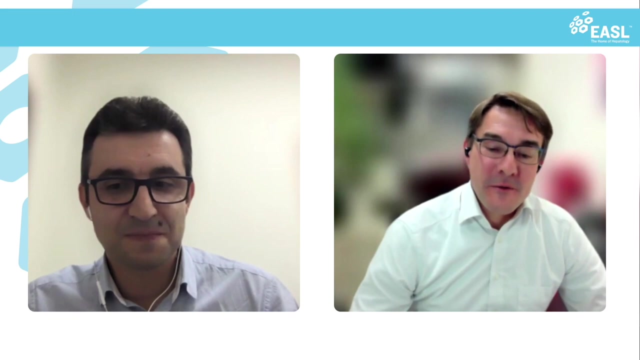 something palpable, something crystallized that patients actually know that this is the therapy will give you if you have chronic liver failure. so what's your view on this? yeah, thank you, peter, for setting up the field so nicely. um, i think, um, yeah, so the so the breakthrough of cell therapy was 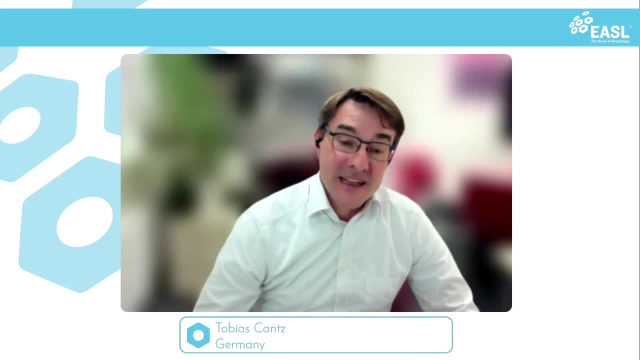 when, when we learned how to cultivate um liver cells and pesticides, at least for a short term, and to to isolate them from the liver and being able to transplant then via the portal vein into to the liver, and i think there we have a kind of a spec special um. 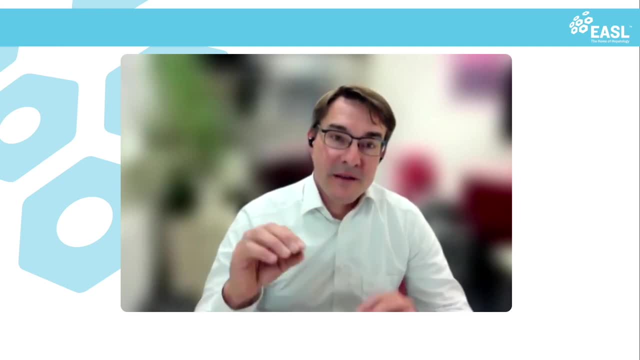 history architecture in the liver, where we have the portal vein that then terminally branches in into the liver sinus. so it's um, where we have an, an efferent vessel that brings cells into the power and kind and through the, the fenestrations of the liver sinus. so it's the, the hepatocytes. 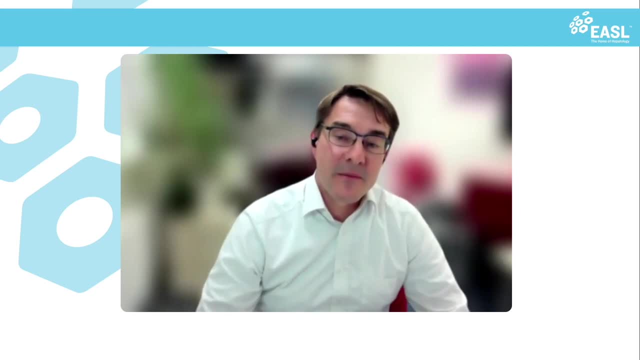 isolated, the pesticides can basically squeeze in the parenchyme and then can repopulate the liver. so i think this was done in animal experiments of course first, and then in a few patients and um. despite, let's say, the metabolic so success, when these cells were transplanted um, one had to realize that it's very difficult to get. 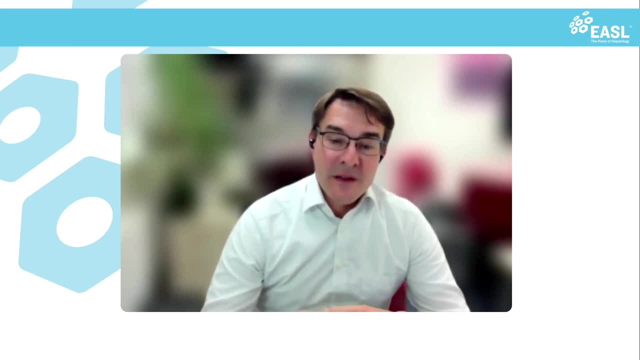 enough cells into the livers and i think one of the bottlenecks still is that that we can probably only provide a smaller percentage- you named like three to five percent, which is one of the goals that can repopulate the liver by this approach safely and this will only help a few patients. 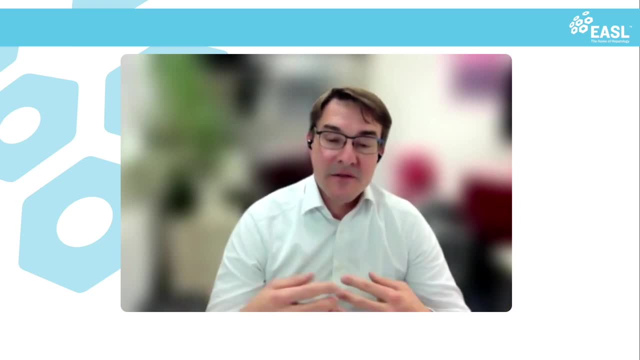 maybe those with metabolic disorders, where the transplanted cells will have the net polar advantage, or some other disorders where only, let's say, a small um, a smaller, let's say, a level of enzymatic activity is needed- but it would be difficult to replace the full liver with this approach- and, of course, the cellular transplants. they are also prone to immuno rejection. so we face the same, if not even worse, immuno rejection problems than compared to the full organ transplant, and i think that the latter is one of the most bottlenecks in in liver cell transplantation approaches if it comes to that, the hepatocyte transplantation. but we have to. give immunosuppression, it's difficult to monitor the small cellular transplant and so those pediatric patients that need to receive such a therapy, they are just better with a liver transplant and i think it's time to acknowledge and the surgeons for the we have a regimen where we wouldn't need immunosuppression for liver cell transplantation. 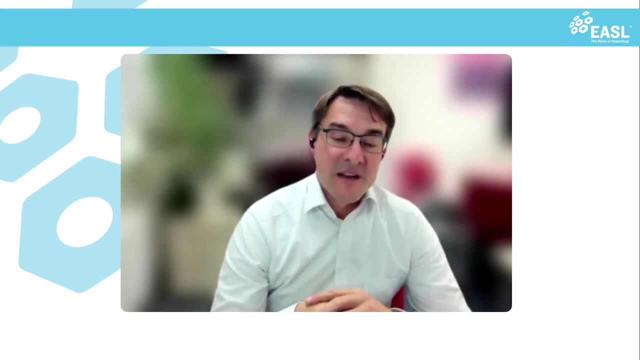 transplants. there might be then the flipping point where cellular transplant might be better, and so this is basically hereditary diseases, where the liver cell transplant would basically be something like a gene therapy. and again, there we have also the competition with the non-viral gene therapy approaches emerging right now. there's also therapies where we just want to kind of fight. 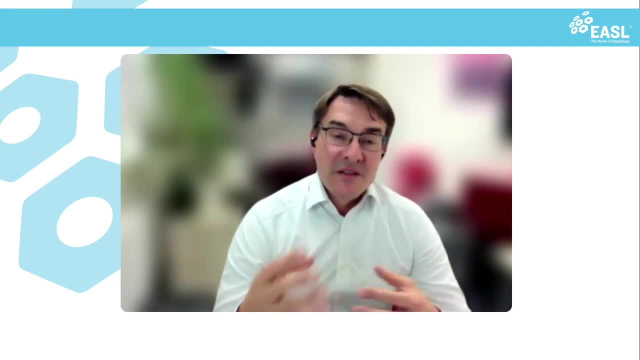 liver injury, liver inflammation, liver fibrosis with these other cell types. so mesenchymal stem cells, progenitor cells, has been discussed to be one of those sources which which strong anti-inflammatory, pro-regenerative function. there's quite some, let's say, clinical work ongoing there. I'm not so much in front of these. I'm much more fan of, let's say, more. 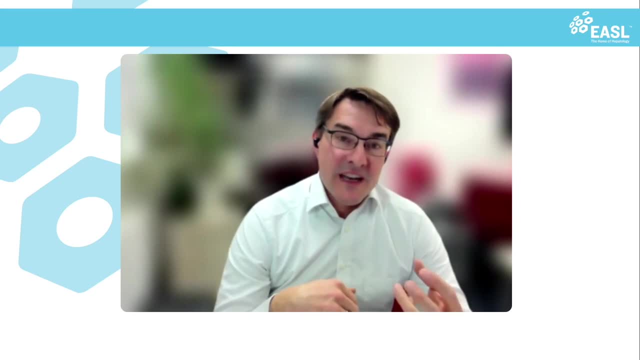 targeted approaches. their immune modulatory macrophages or better defined cells can be used to fight liver injury, and so I think that's a really good point, and I think that's also one of the future directives to us- to understand a cell therapy not only like a gene. 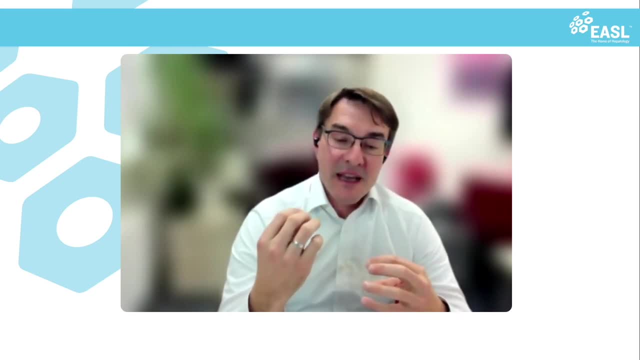 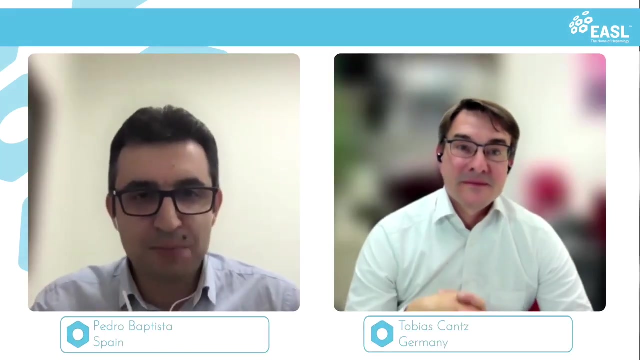 therapy approaches where a defect metabolic enzyme is replaced, but also as an anti-fibrotic, co-regenerative approach, this immune modulatory cells, and I think there's also a lot of things that we will know in the next upcoming years. so that's thank you for that, because that's. 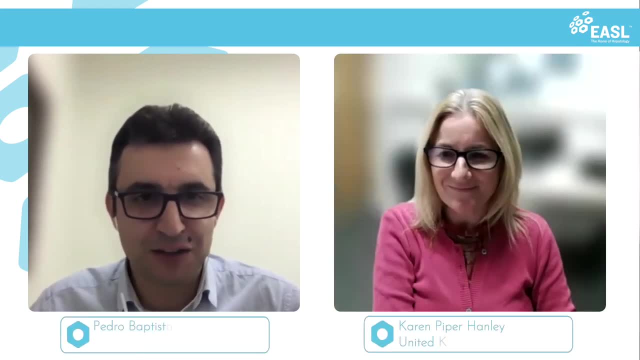 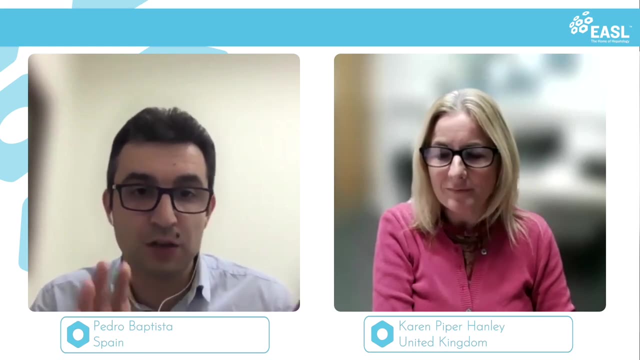 actually where I want to pass to Karen as a specialist in fibrosis. so I mean, there's there's already out there quite a lot of clinical trials. some are more limited in their scope: a few patients, but with some of the different cell types, that to be as 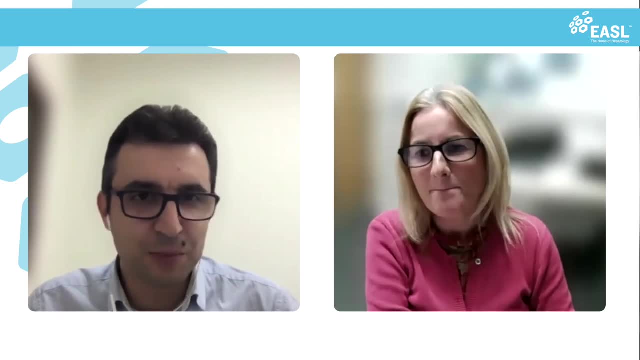 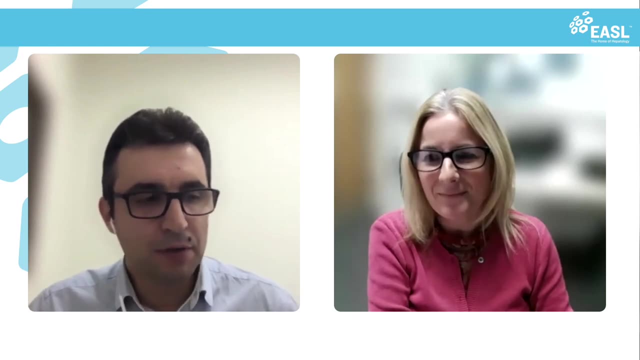 just mentioned. I mean fibrotic environment, inflammatory environment is is really a nightmare if we think you know how to treat it. but so how do you see this coming? because one of the things that I see is that a lot of of these clinical trials, particularly some of 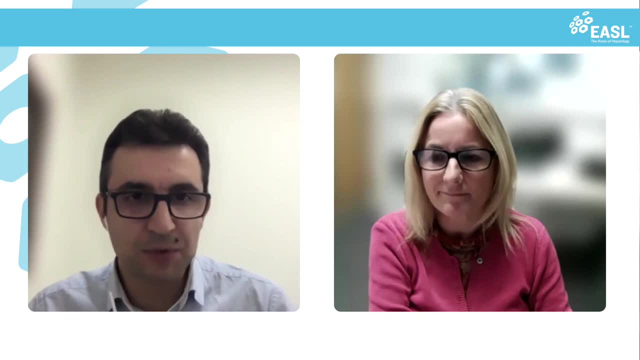 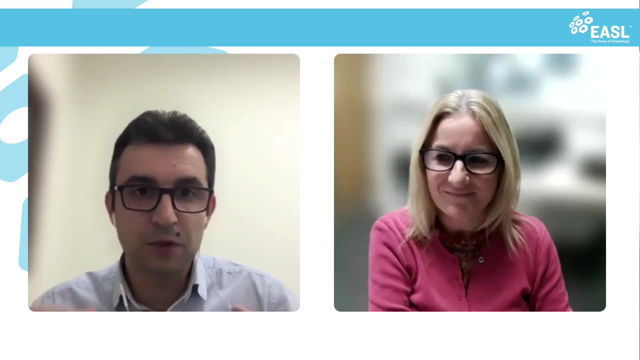 with MSCs or even, like with some of the macrophage. sometimes they are actually contradictory. so some say that there's some effect. some others do not show any effect. so how do you see this from the perspective of what we know about fibrosis and fibrosis regeneration, which is what we don't know? 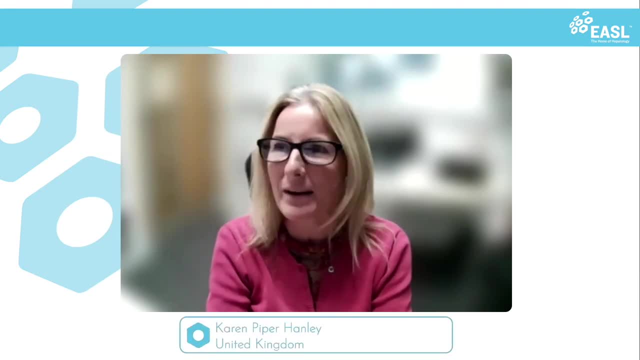 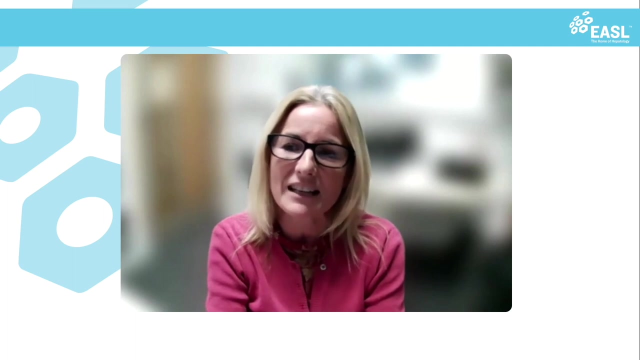 as much. if we want to start addressing that, we should think about, you know, the kind of classical understanding of how fibrosis manifests, and you know, I guess what you would naturally understand is that there'd be some sort of injury with inflammation that would activate a kind of an epithelial cell and in liver, classically that would be hepatic stellate cells, which become proliferative. they migrate into the, the hepatocytes and cause damp tissue damages. they, they lay down matrix and cause a scar and of course you know we haven't thought about, you know how, fibrosis. 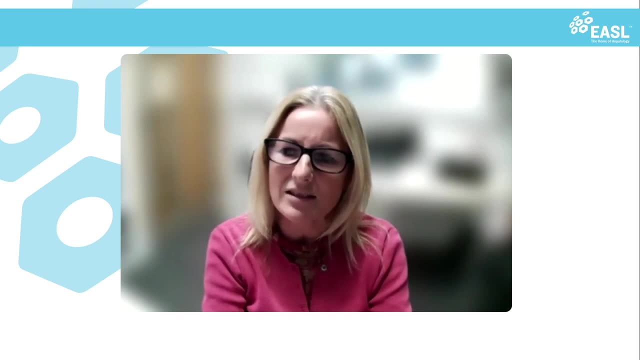 progresses and we made such great inroads into this in terms of understanding hepatic stellate cells and and how they kind of lay down, matrix, the signaling pathways that influence this proliferative response of stellate cells. but I think what we're now coming around to- and you, you touched on it beautifully at the start, Pedro. is that actually it's a failure of regeneration. so not only do we have this kind of scar and response, we also have all of the cell types surrounding the scar that are also involved and, in terms of this, this idea of an impaired damage response, impaired proliferative response of the kind of hepatocytes and cholangiocytes. 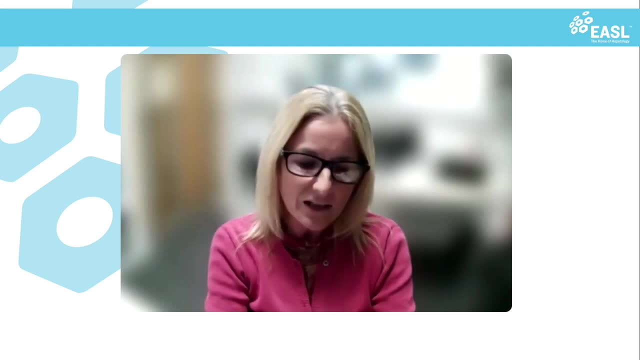 I think that's becoming much more widely accepted. so, in effect, fibrosis isn't down to one cell type of people. as you've already said, it's down to multiple cells that are involved in this kind of pathogenesis, and so how we go about targeting this, I think there are multiple sides of it. so 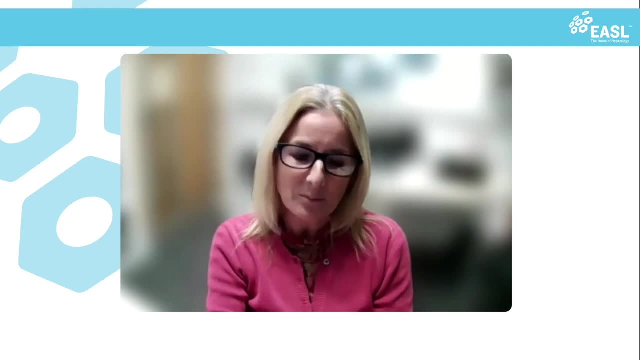 we need to reduce inflammation. that's absolutely critical, but also, given the massive amount of information regarding how stiffness within the liver can influence and modulate cell state and damage within the liver, I think we also need to reduce scar, and so we need to look at both- modulating inflammation, modulating scar- and be that through 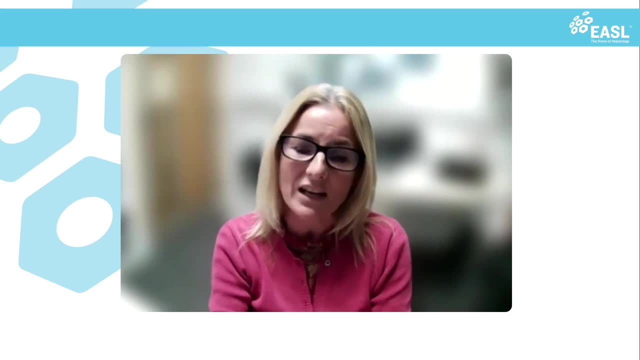 reducing stellate cells or somehow breaking down matrix. And then, thirdly, we need to understand how to improve that regenerative response or repair the regenerative response that's gone wrong. and I think you know that's something that is now becoming much more prolific in the fibrosis world because of the the advent of single cell. 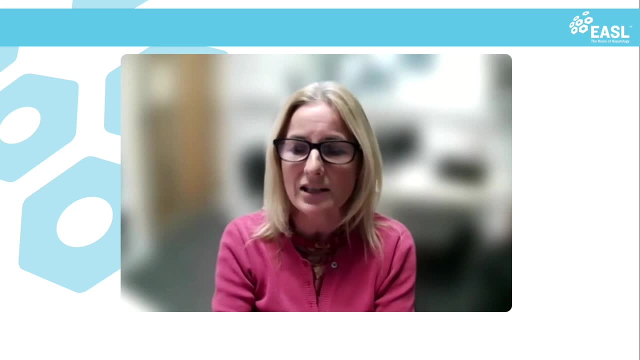 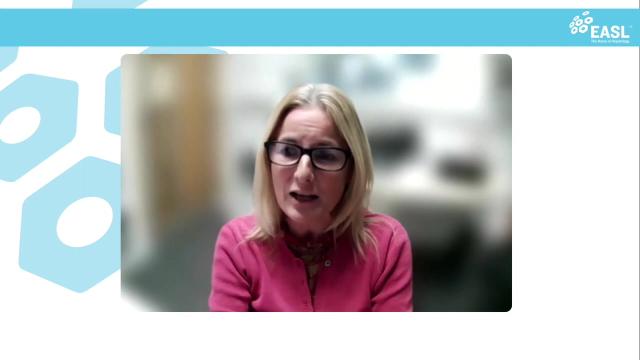 technologies and certainly with spatial localization that allows you to really see where these kind of impaired responses in the liver are happening, directly in response to the pathophysiology. So I think there's quite a lot to learn still, but I do think that there's a lot we can draw from development, because that's certainly 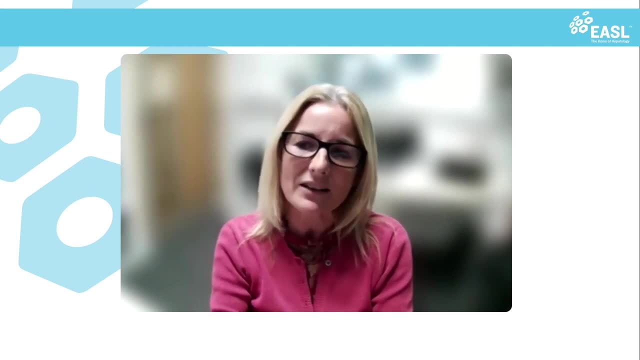 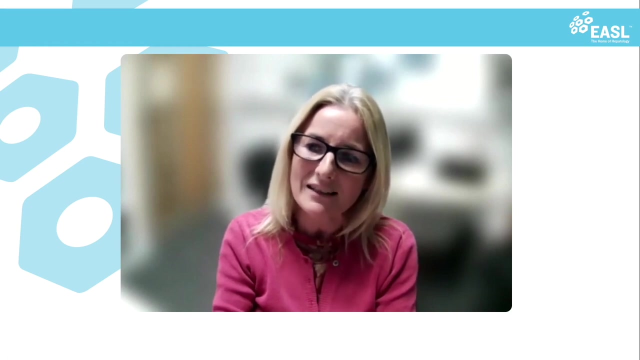 an area of. if we know how the liver is put together normally, then we'll start to be able to pull together all of these kind of new technologies, these new understanding of the impaired cellular response, and say, okay, we can do this and we can do this and we can do that. So if that's part of a normal, normal liver, 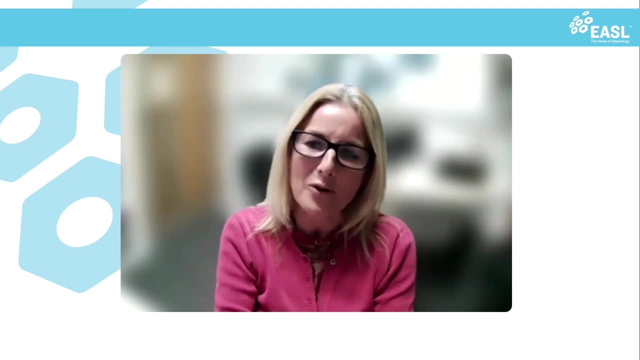 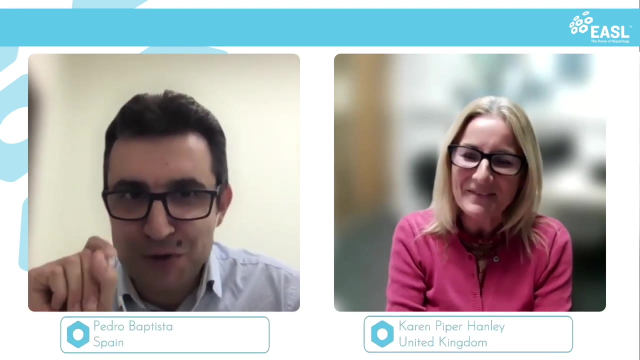 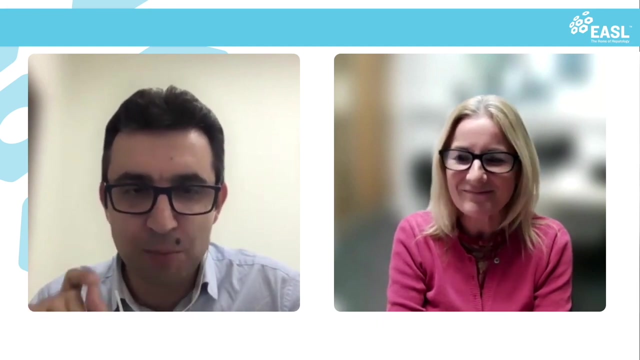 developmental response. can we repair that in an abnormal or impaired response due to injury? So just before I actually take on what you just finished saying, I want to say something that I missed, which is encourage our audience to actually ask questions in the chat, And I'll promise that. 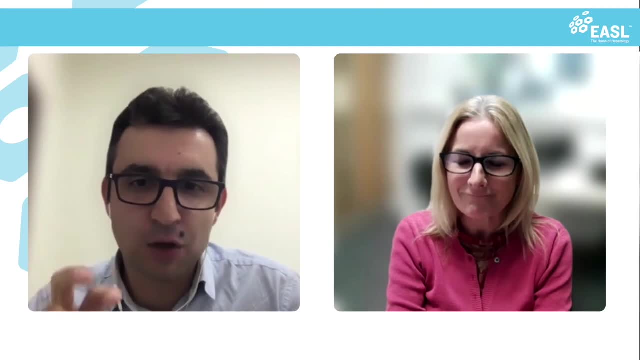 all of them will be answered, even if they are not answered in within the session. we'll post this within with the episode once it's edited. but now, picking on what you just said, which is the developmental biology, i'll just pass this to our specialist professor lemager frederick. 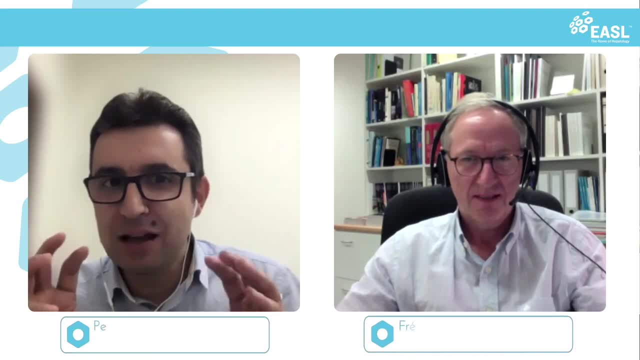 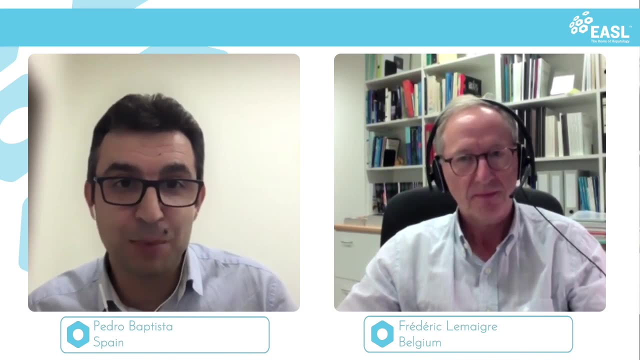 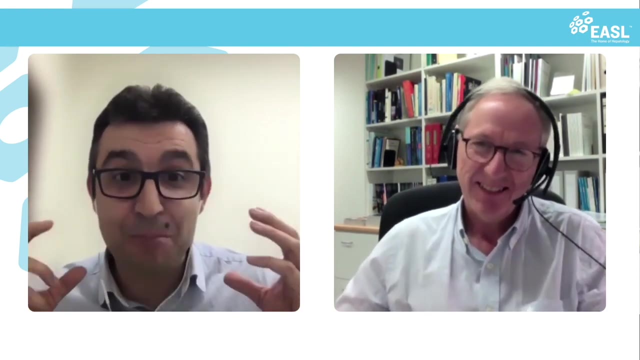 so how do we so, taking into account that a lot of the levers we're going to be repairing or that we want to regenerate are fibrotic? how do we do developmental fiber developmental- see, i'm already even catched by the word. so how do we do developmental biology in a fibrotic scaffold? 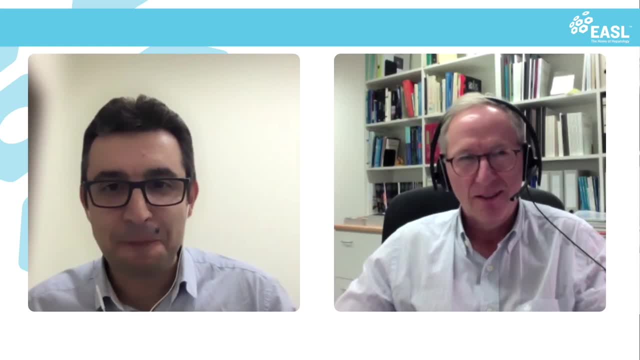 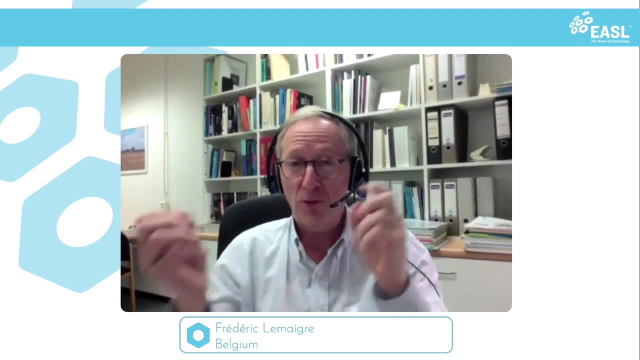 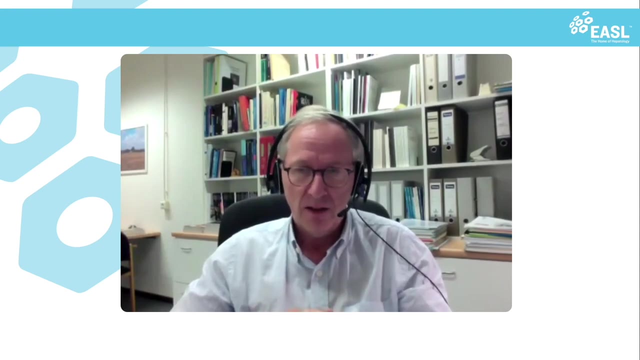 or in a fibrotic environment. so that's a particularly difficult question, because we are going from a wrong perturbed environment and we are supposed to go to recreate a correct one. so what developmental biology can bring about is to understand at least how you can go to a normal. so you first have to define what is a normal. so you first have to define what is a normal. so you first have to define what is a normal cell. and that's already not so easy and and most of the work in the last 25, 30 years in. 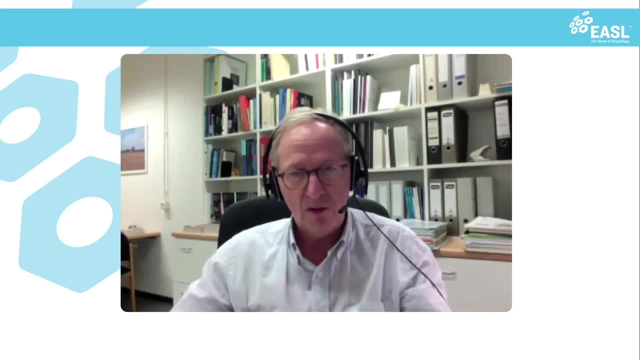 developmental biology of the liver has actually been focusing on how you go from progenitor state towards an adult, mature state and, and here again the focus was essentially on hepatocytes and cholangocytes. i'm not saying that other people have not studied other cell types, but when you look at it, um and you, you just go to pubmed and you type development of 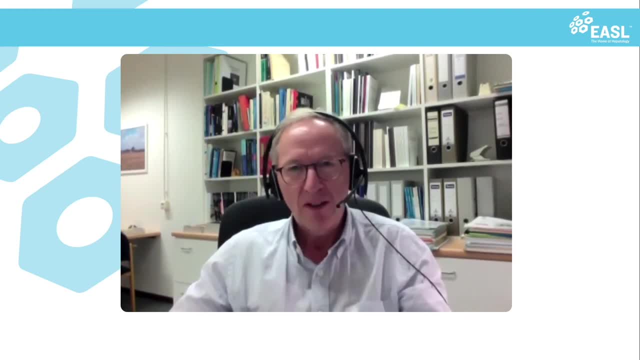 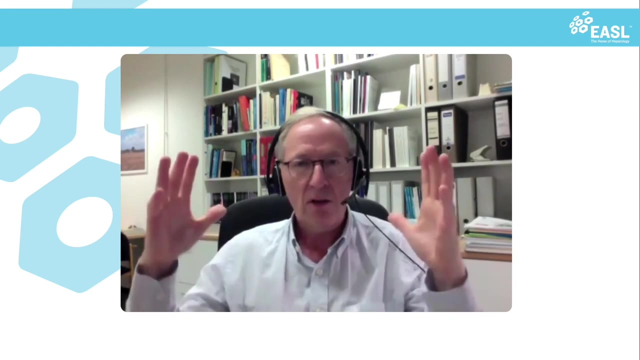 stellate cells. you know you don't find so many papers um development of the mesenchymal tissue in the liver is is clearly understudied um recently people, for instance, have been focusing lots of attention on single cell rna sequencing analysis. and there you see, you know lots of data like that. 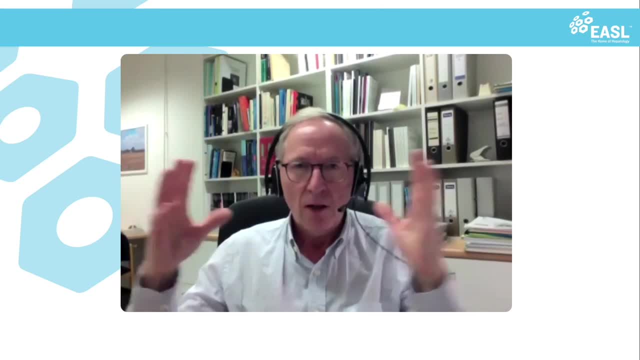 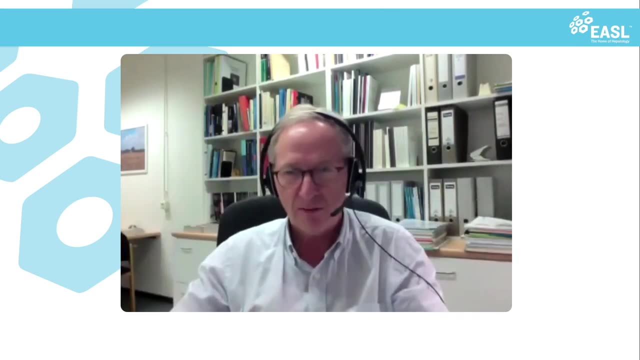 on hepatocytes and the telial cells, a bit less on cholangocytes, because the cells are not numerous. and then you see it, you know a few spots and these are all the mesenchymal cells of the liver. yeah, and you dig into the data, you, you don't figure out what it all is. so we have and, and there is a huge 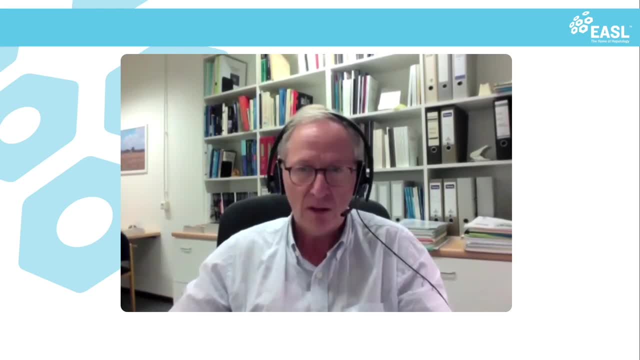 gap in knowledge in in development of the mesenchymal cells which play around, play a role in in in fibrotic diseases um and um. my feeling is that developmental biology over the years have has has um generated lots of information how to um generate mature or, you know, close to mature, cholangocytes, hepatocytes also at some degree. 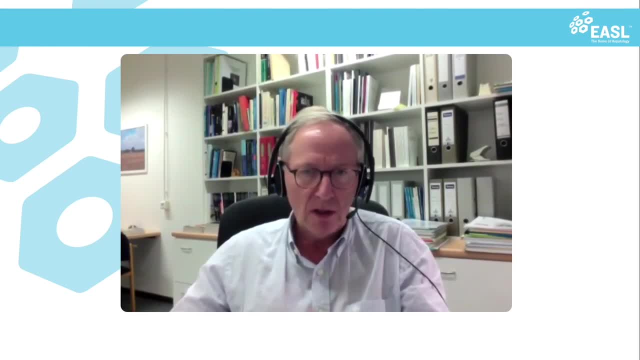 endothelial cells as well. but what is critically missing is what is being done in in the non-epithelial cells, that's, that's a major limitation of the study. and what is also critically missing, in my view, is is how those cells interact and are connected to each other. so, pedro and i for 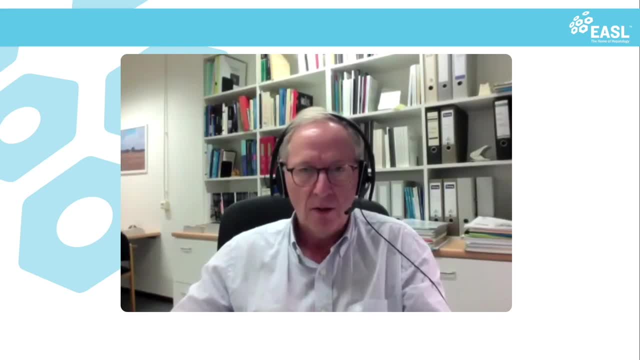 instance, have been discussing together. uh, a very simple question. we have hepatocytes, we can generate hepatocytes, we can generate cholangocytes, but nobody can bring them really together and nobody in the developmental biology world can tell you how the two cells connect actually during development. so we can generate 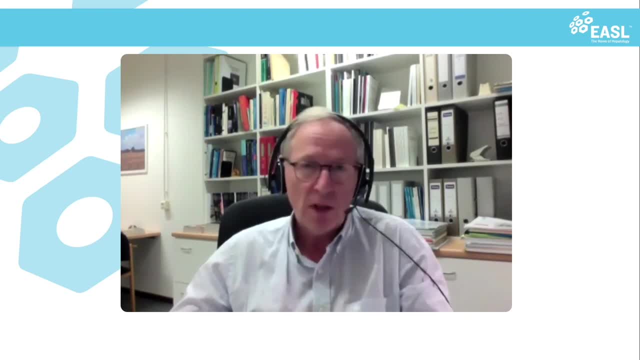 cells. we are missing a number of cell types and we and we cannot even connect them all together. so what can we do except, you know, relying on some pre-built structures? like you know, pedro, pedro, you are doing these kind of things, you, you, you start working on decelerized liver, but what? 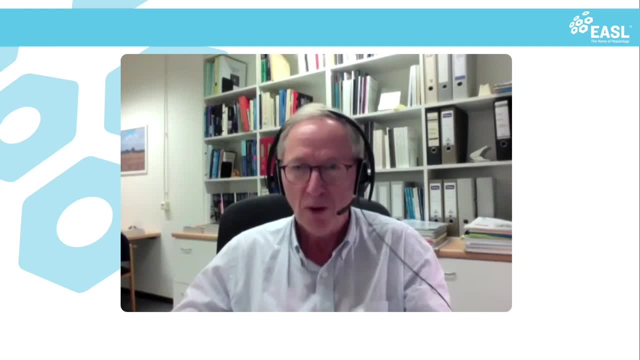 you're doing is somehow what the developmental biologist would not do is to start with a pre-built structure and then try to fill in the cells, because that's not how developmental biology occurs. but it would be one way to circumvent the limitations that developmental biologists 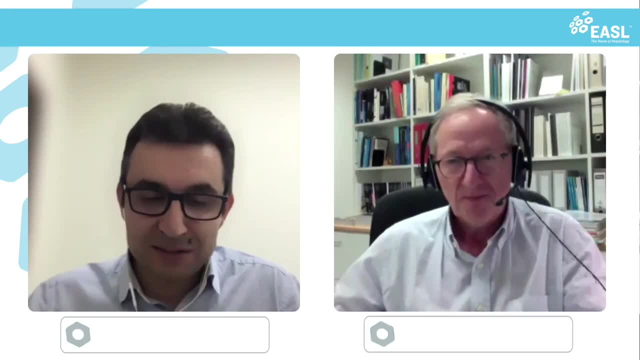 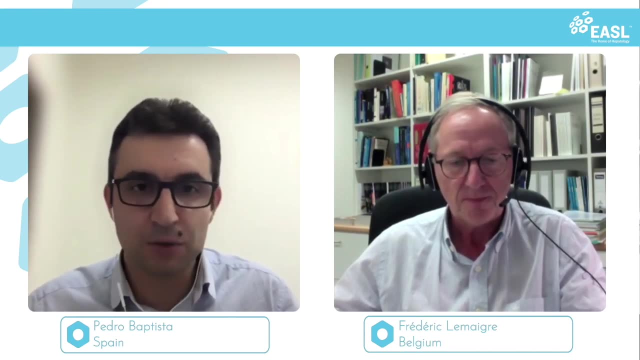 have so far not uncovered yet. so taking on that- i mean that is also one of the focus of our consortium- and regenerative pathology, which is, if we are able to generate bioengineered livers for transplantation, then it doesn't matter the size, because you can kind of tailor that if you need. to substitute just a metabolic function by five, ten percent of the function. pretty much like what was attempted in the clinical trials with hepatocytes and msc. so small amount, five, ten percent size. or if you actually need to just do an orthotopic transplantation and taking. 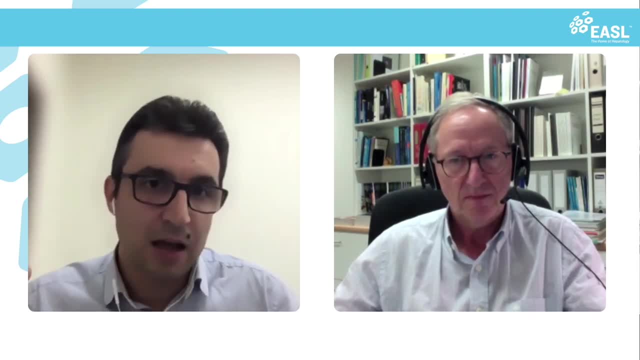 a fibrotic or cirrhotic liver out and then put i wouldn't say a hundred percent, percent liver mass, because i think from the bioengineering point of view that's still massive. you're talking about hundreds of billions of cells, but at least 30, 40 percent, whatever mass can. 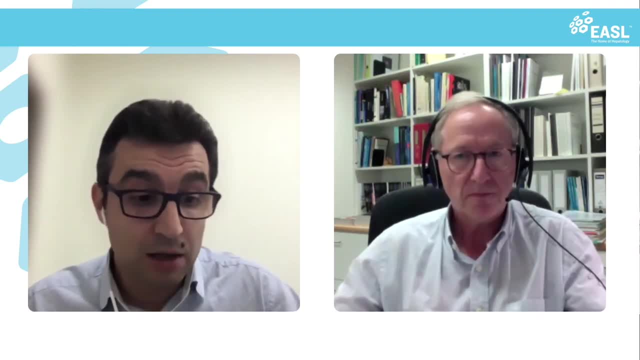 provide the function to keep the patient alive. so in that regard, frederick, i, i completely agree with you. i mean, i i think we have made big strides in the last decades in developing some of the techniques, getting some of the cells with really high quality, being those primary or es or ips. 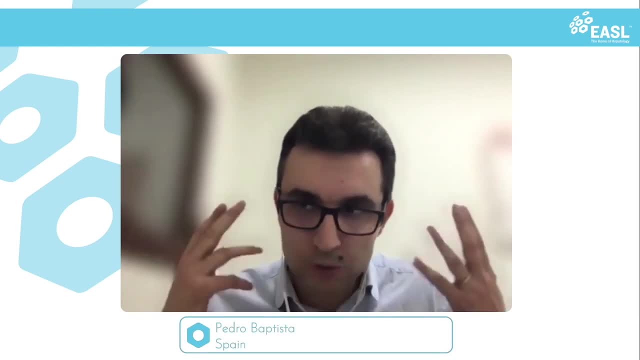 derived. but what we have not made is that we have developed some of the techniques, we have developed some of the cells with really high quality, being those primary or es or ips derived. but what we have made is really, when we're trying to address the problems of hepatic tissue generation, vascular 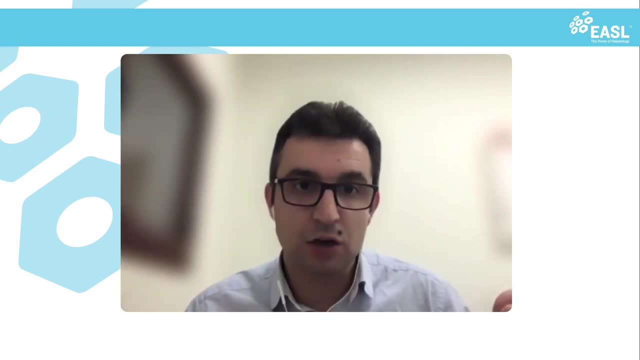 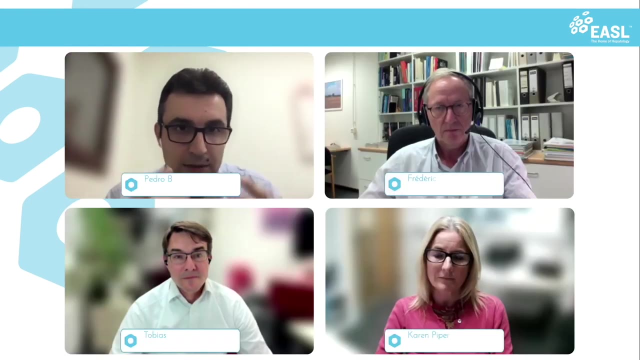 tissue generation, biliary tree generation and then full integration between all these different tissues and and vascular trees in the bioreactor, in these scaffolds. this is still what we don't know, because this is really trying to replicate the developmental biology mechanisms in vitro in a bioreactor in a way where that is still kind of unknown to us. i i can add that i 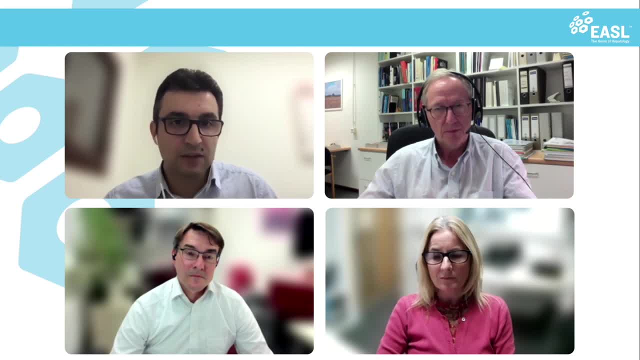 i, i, i think, since we're now able to actually get some of these things together and have this template of this cellarized liver scaffolds. although this is not how developmental biology happens, this is an interesting tool because you're forcing the cells spatially to get together in 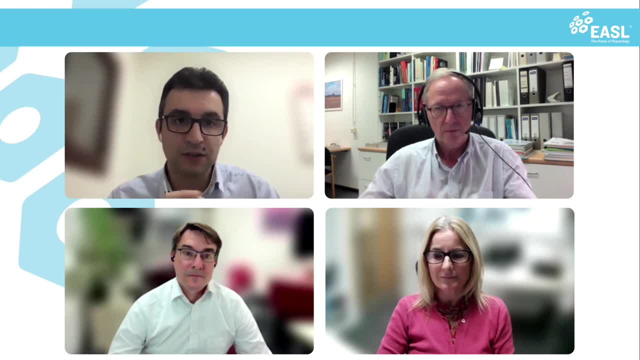 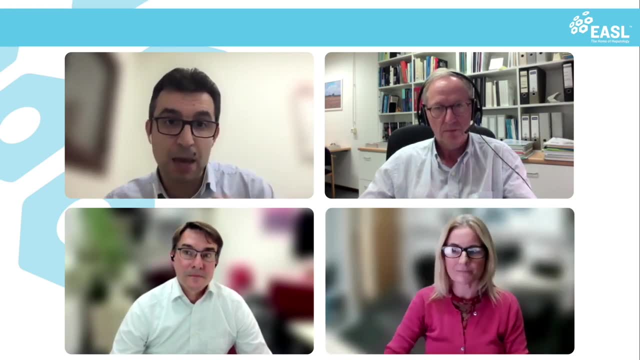 certain spaces, because this is what we can do as bioengineers, is localize the cell stores, certain areas, and distribute them depending on different percentages, so you can localize hepatocytes and cholangocytes and the endothelial cells and and the endothelial cells and the endothelial cells, and 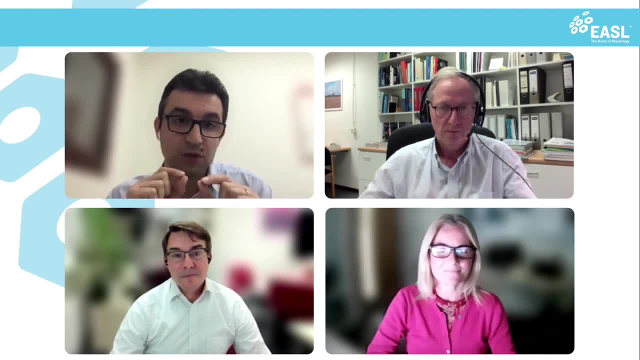 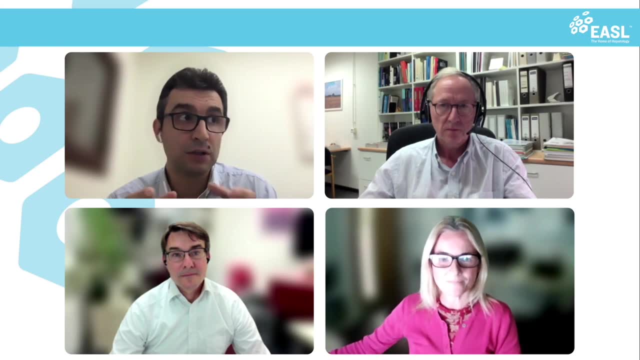 chlamydia, and the endothelial cells and and the endothelial cells and and the endothelial cells and cell stores, the whole parenchyma. but since you infuse them through different places, so you're going to force the interactions. but then this is, like i said, i think, an interesting tool, not only. 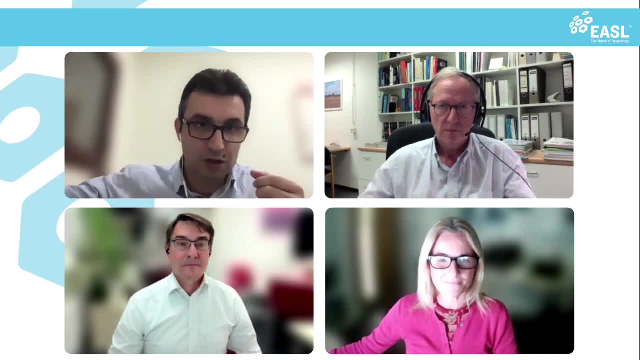 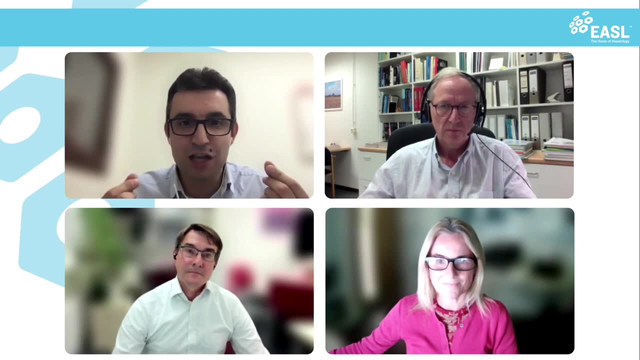 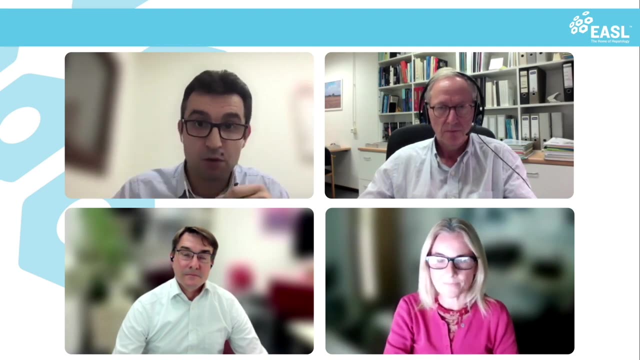 good for the bioengineering of the future livers we want to transplant, but also, i think, for just, you know, the nitty-gritty developmental biology in human cells, when you actually put all this together in the bioreactions and then you try different mechanism inducing different growth. 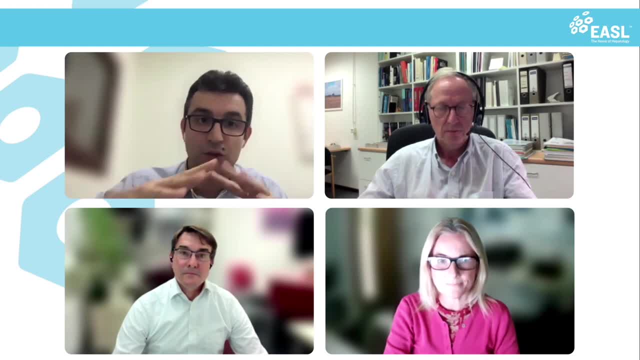 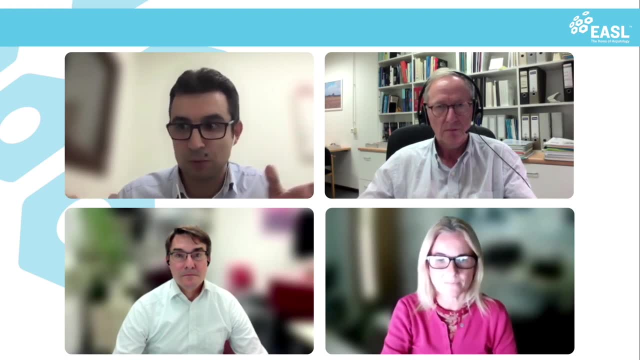 factors, etc. and see what happens when the cells are trying to interact together. so this, this is, i think, something that that is, the current knowledge of what we have to to do the bioengineered livers, but taking this further to all the scaling up that we need to do for the massive, large-scale. 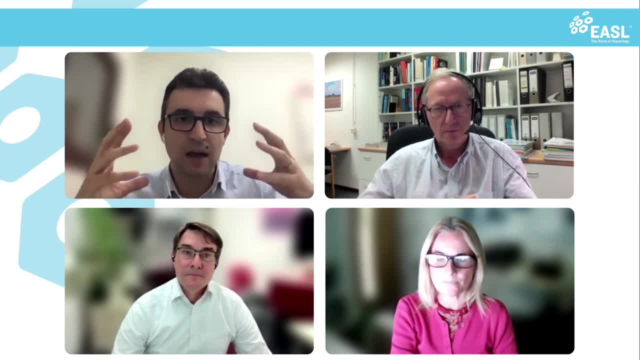 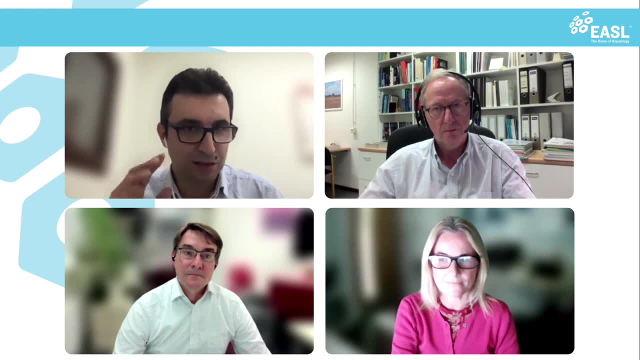 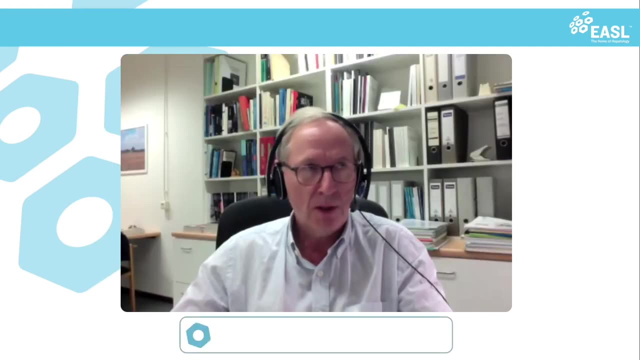 cell expansion and then integration this into meaningful size bioengineered liver. so it's still something that i think it's, if not decades away, still a lot of years away. yes, at the same time we are we are facing some kind of difficulty because- let me give you an easy example- developmental biologists in the past have demonstrated that. 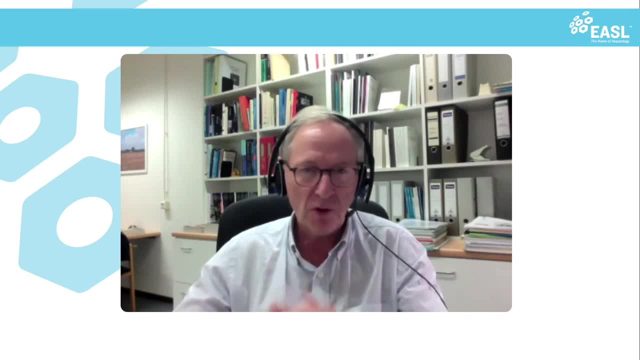 hematopoietic cell in an embryonic liver secrete oncostatin m, and this oncostatin m then promotes differentiation of the hepatocytes. this turned out to be relatively easy to replicate in in two dimensional cultures of stem cells. so you put oncostatin m and the differentiation of the 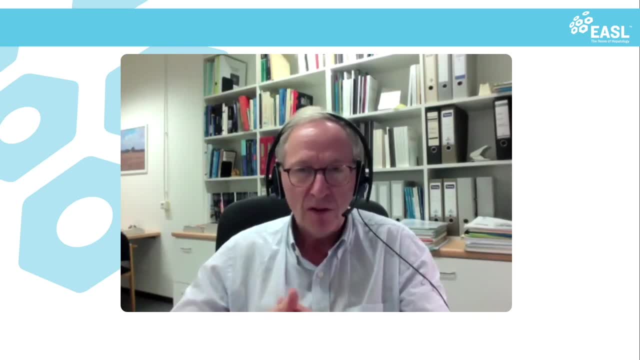 hepatocytes is improved. but but now we are facing another difficulty: how would you do this in in three dimensions? coming back to, you mentioned that the uh, the biliary tree. well, you know that in development, the biliary tree sends signals to the mesenchym around it and so shapes the 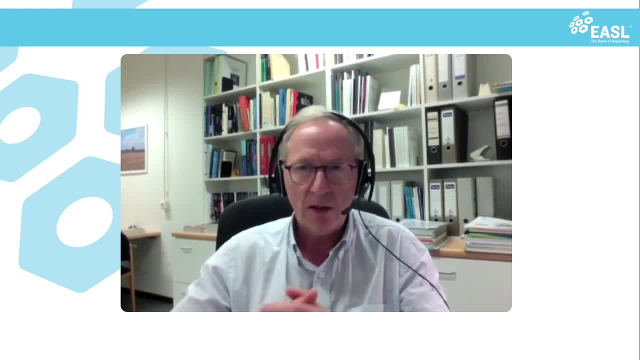 mesenchym, and so shapes the uh- the structure of the hepatic artery, and and so also shapes the uh- the presence of various cell types. um, here we are facing a difficulty. this three-dimensional difficulty is something where developmental biologists have not been able to truly help the bioengineers at this moment. that's one of the major challenges for us. 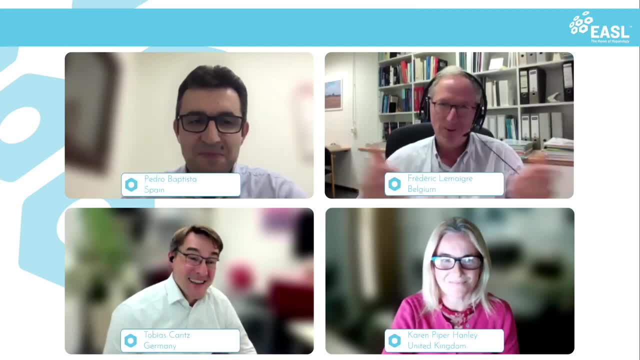 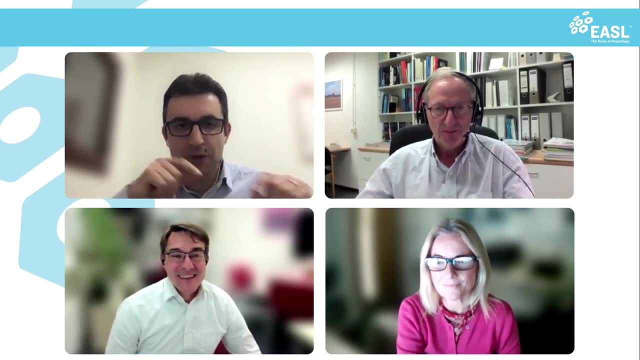 actually it's four dimensions if you consider time. right, no, but, but, but. i i think it is happening, though, because the fact that we can now try to understand the interactions and the cross-talk that happens between these cells, being this in the mouse models or in this organoids 3d- 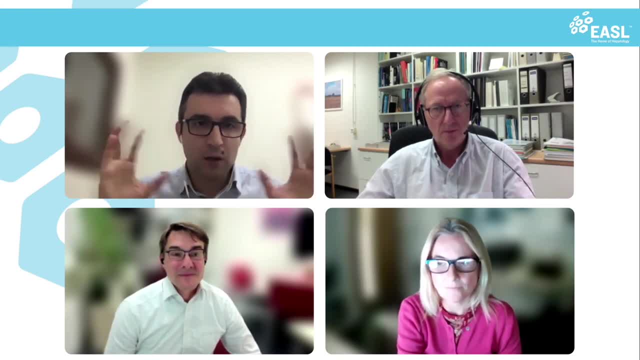 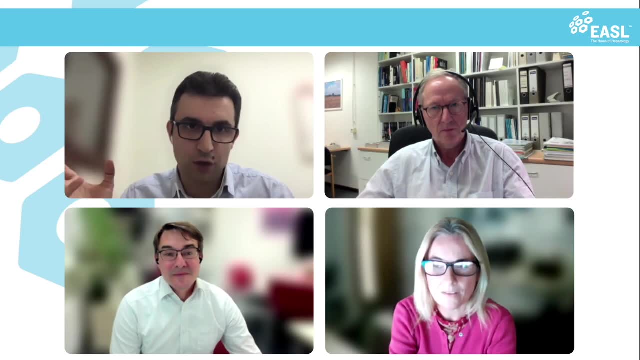 models, bioengineered liver models. i think it will. it will really provide us in the next years a wealth of knowledge that might really be helpful in this final quest of, uh, bioengineering a liver that we can transplant. but but there's one thing that i think it will be helpful- not only to tobias, for 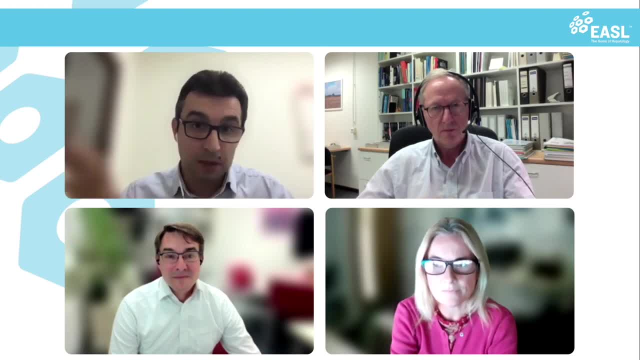 for the stem cell or liver cell transplantation, and to also you, frederick, and me, which is really how to understand how all these mechanisms of fibrosis, or pro regenerative mechanisms that need to be activated in the livers, actually help if we actually take together- and this i'll pass to karen- what's happening now with 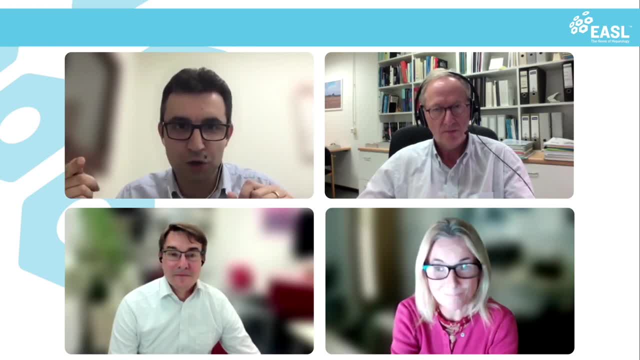 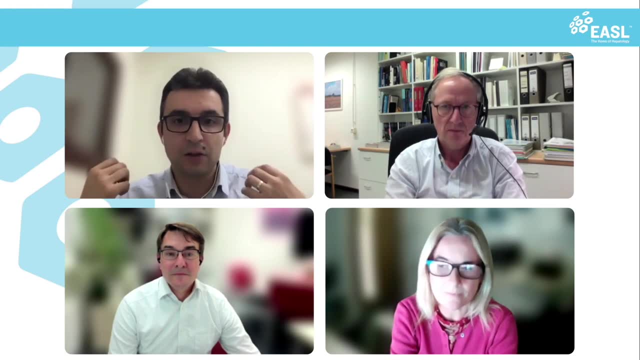 hepatitis c positive patients that actually got cured of the virus, that had already fibrosis and that in certain cases we are actually seeing there are regressing in the level of fibrosis they have. could this be actually the forever trove that we need to understand? how do we actually heal? 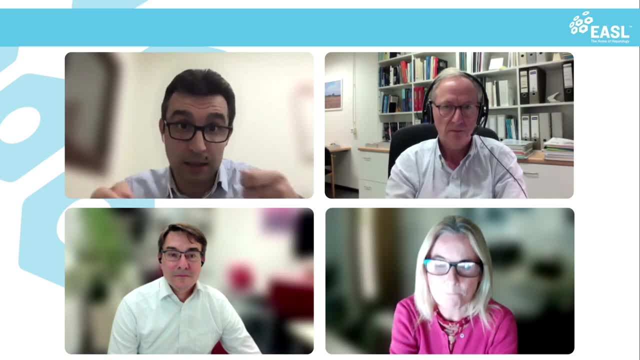 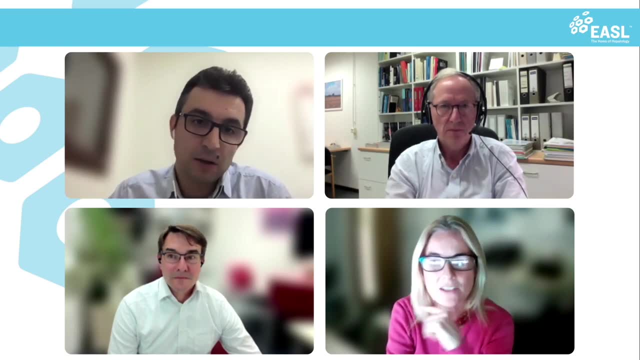 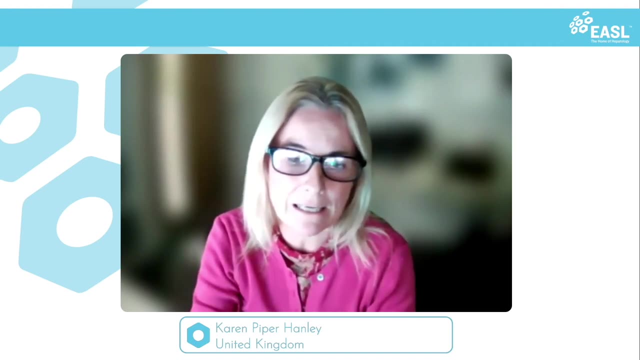 the scar tissue, and then we can try to do something about regenerating further a parenchymal tissue that was damaged, i think. i think the hepatitis c story is really interesting, though, because um so, so you know. so. so hepatitis c, um, again, it depends on the progression of the 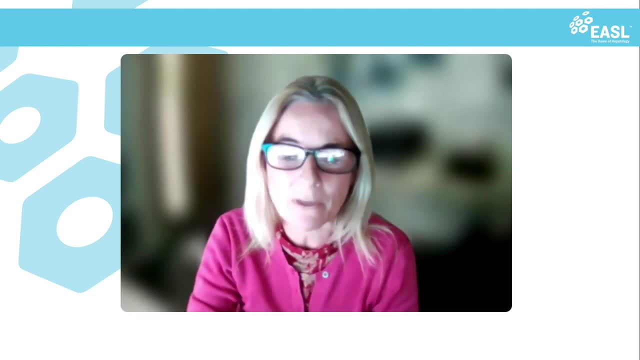 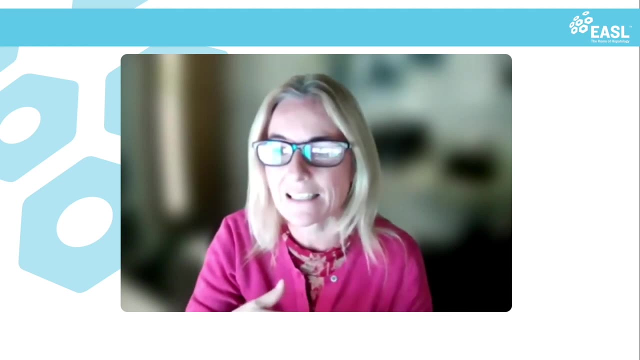 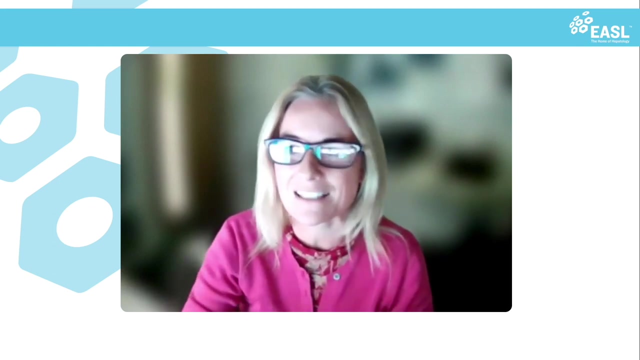 disease. so you know, um people who, who had got hepatitis c and had developed a certain stage of fibrosis. so classically, and i get, i'm not, i'm not a clinician, but we've done quite a bit in this stage and would be, you know, a staging of six different stages, wouldn't it? so six would be. 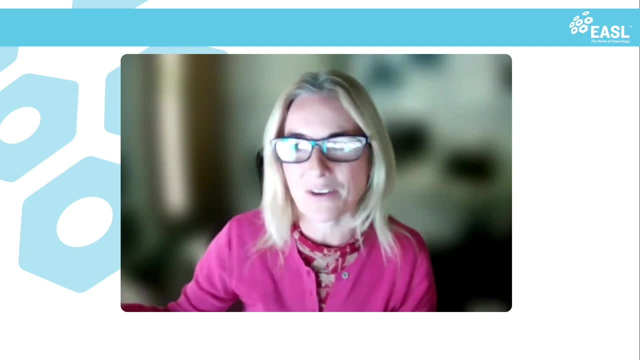 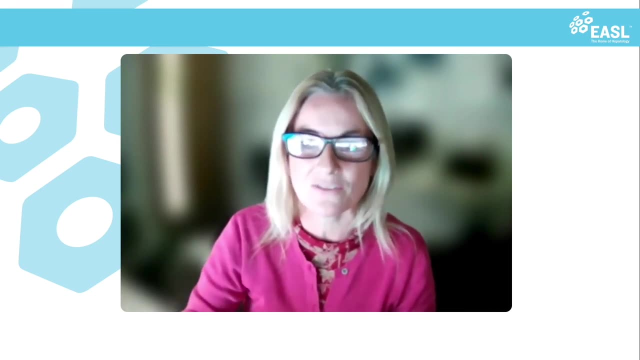 cirrhotic and one would be a very mild fibrosis. so i think what you know, what we shouldn't get mixed up about, is the fact that if you're in that sort of stage three, stage four, even, then the likelihood is, if you remove the virus, even before these wonderful antivirals, the liver would resolve. 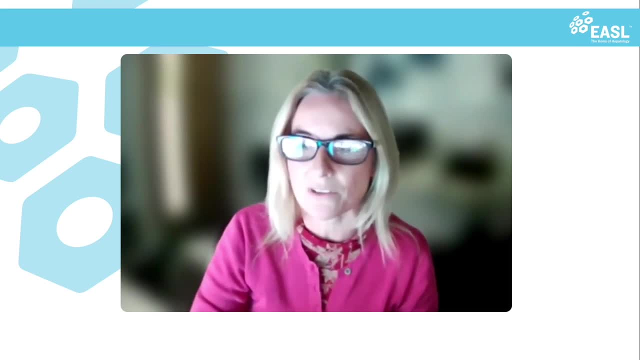 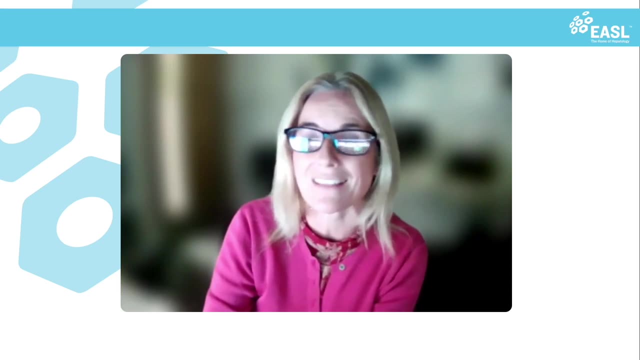 and get better. and so we know that if you remove the virus even before these wonderful antivirals know that, we know that that works and it would fully get better. the problem is if you'd then gone beyond that point and whatever that stage was, or you know whether it was some genetic- 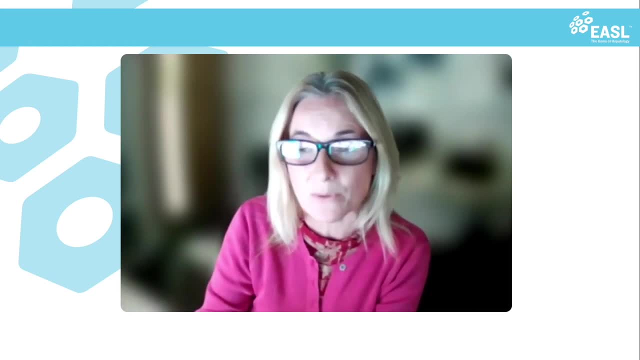 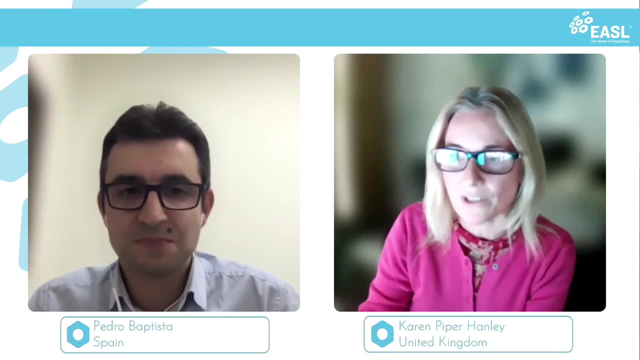 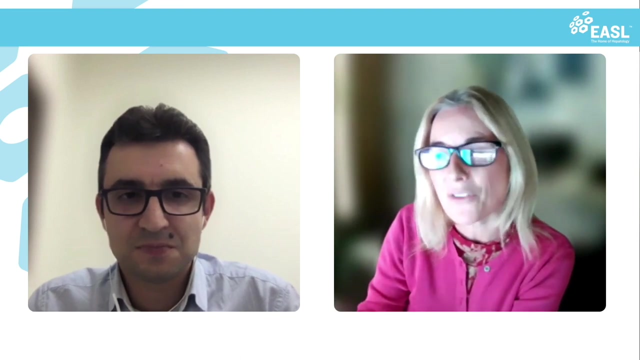 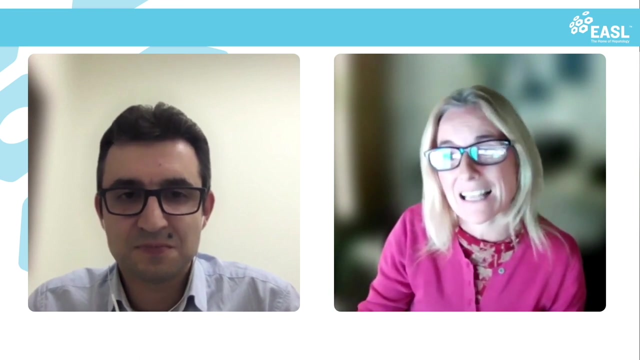 contribution from a, from the person at an individual level. then even the antivirals that are now there and beautiful and work and completely clear the virus. there are people who have such severe liver damage that it's beyond the point of fully able to repair. so clearly that sort of suggests that the environment. that scar environment, the damage that's there in other cell types, is really important in maintaining that sort of pro-fibrotic response, if you like. so even though you've removed the insult, you've still got damage and in fact you know people who have had. 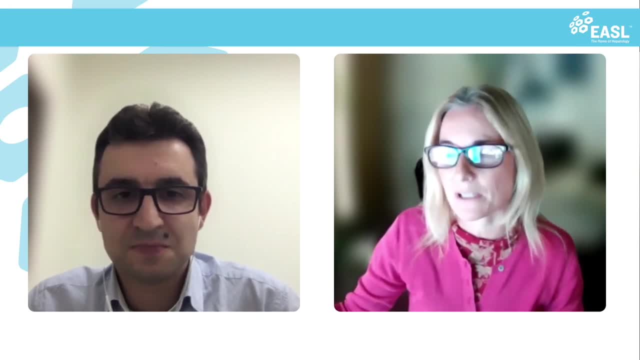 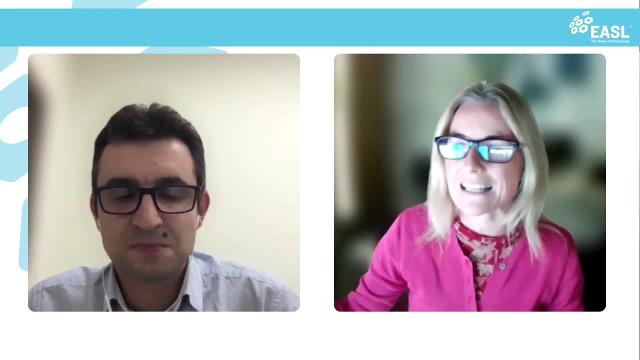 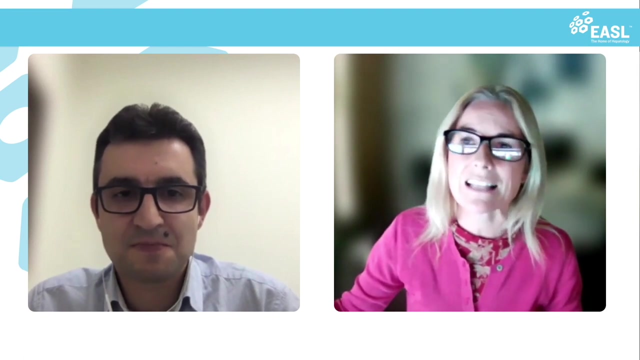 hepatitis c or hepatitis b and very severe liver damage. and even with hcv, where that has the viral load has been completely cleared, they're at a significant risk of developing hcc if they still have severe cirrhosis. so so my worry is that you know we need to work really. 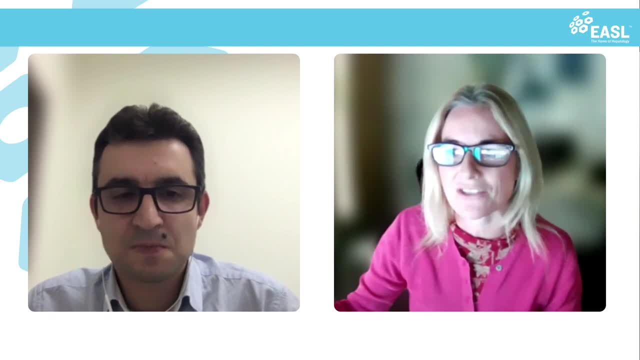 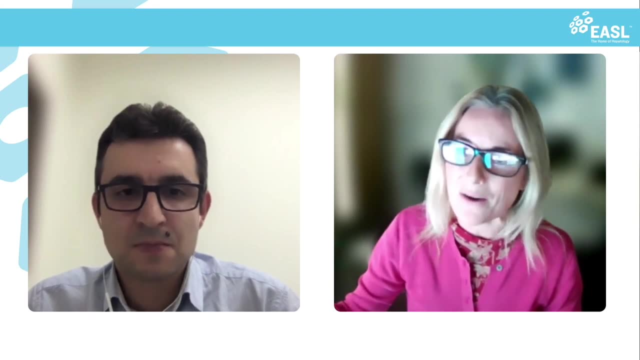 closely with clinicians to understand that progressive nature of disease because, you know, also it's about understanding what's going on in the environment and what's going on in the environment and what. what are we trying to do? you know, how are we trying to regenerate the liver. and most times we're asking a very badly injured liver to regenerate because if it's not, it will regenerate. we know we can, we can improve that, but most of the time it is this severe liver damage that we're trying to ask the liver to repair itself. so so my, my sort of cynical side would say: 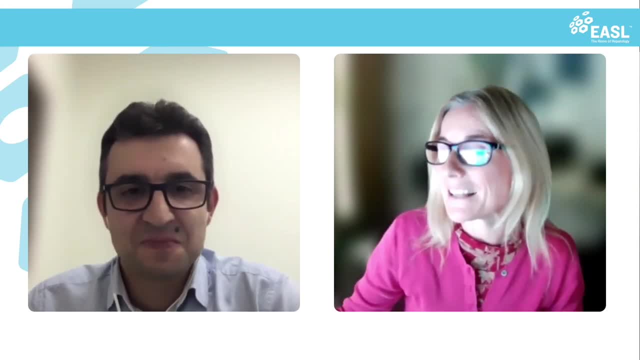 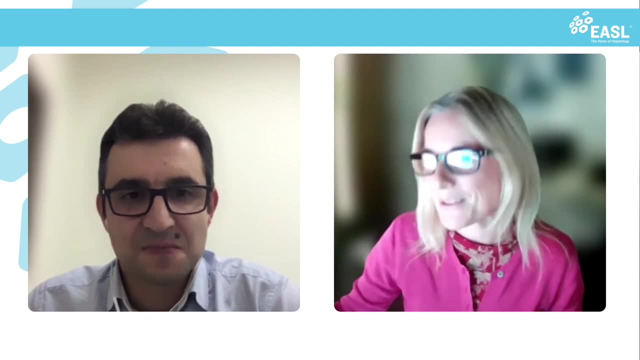 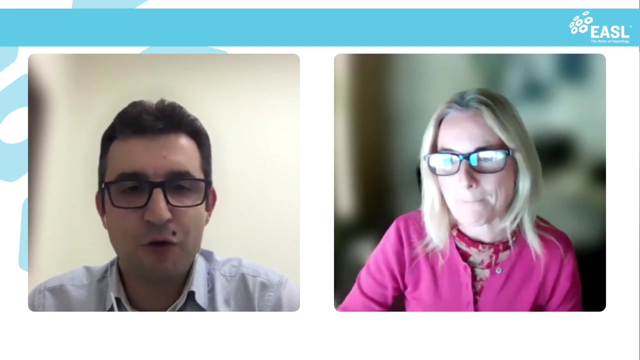 how are we going to improve the way the liver regenerates, or even with new cells, if we put them in the liver at that stage? there's clearly some other other things that we have to get rid of to improve that. so is there a way, then, to say how far is too far, or to determine how far is too far? 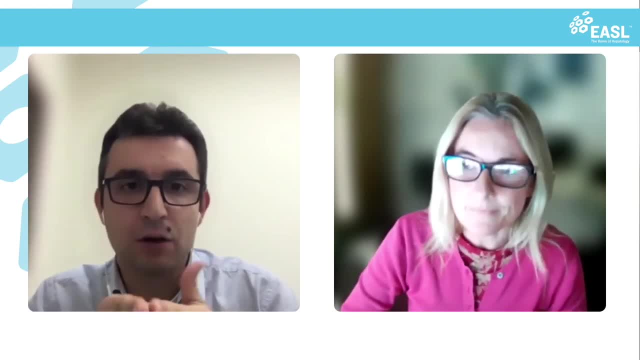 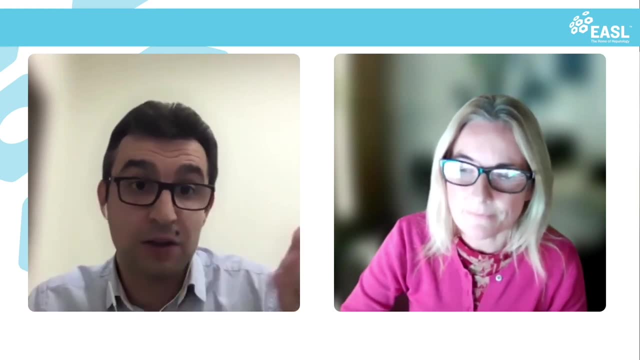 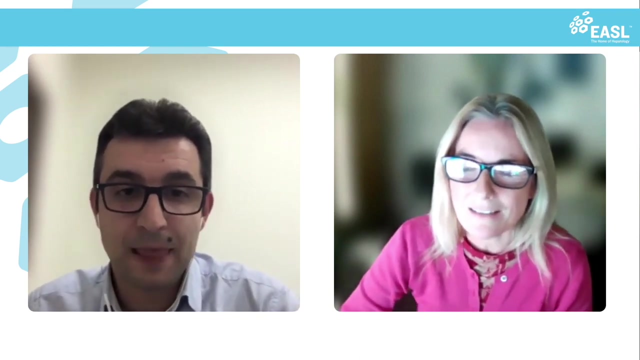 or where is the thin red line of this, can still regenerate and it will be better if we actually help, or this is too far and the only thing we really have available is how far we can go for an appropriate transplantation. so is there a way to know that? do we actually know that? well, i i suspect hepatologists would be able to tell you. 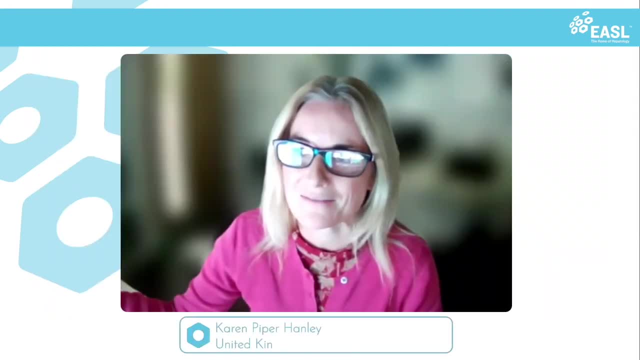 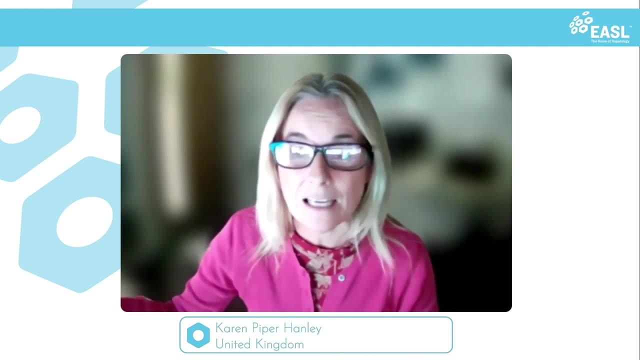 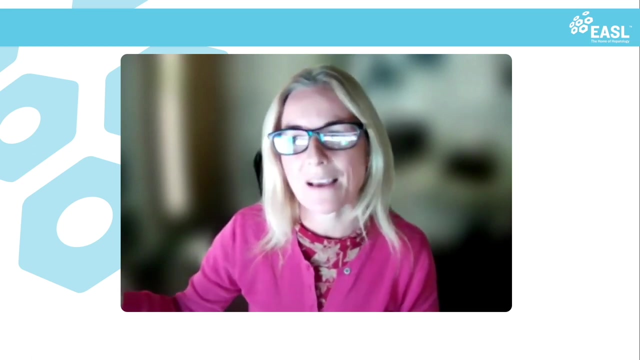 that you know that, that there is a point certainly where there's very little return, very little improvement, and clearly patients are still treated to try and improve liver function, but i think you know that a hepatologist would tell you there is a point where that becomes less effective. 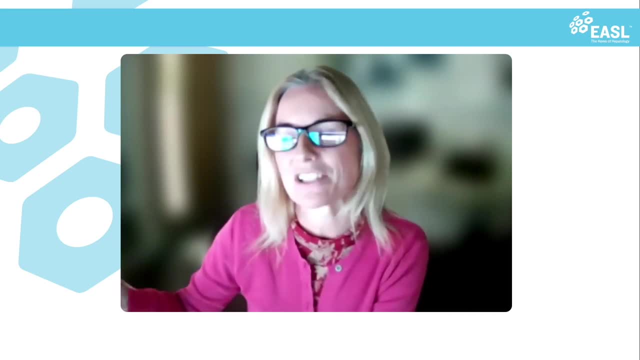 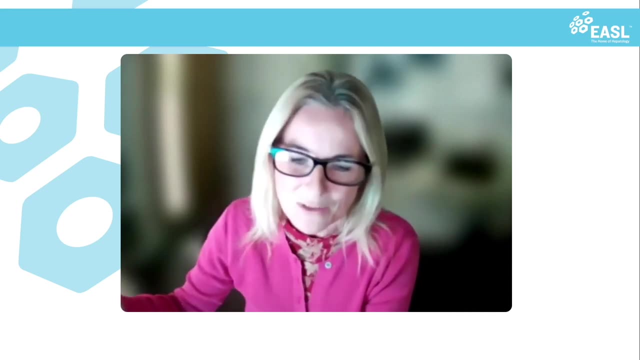 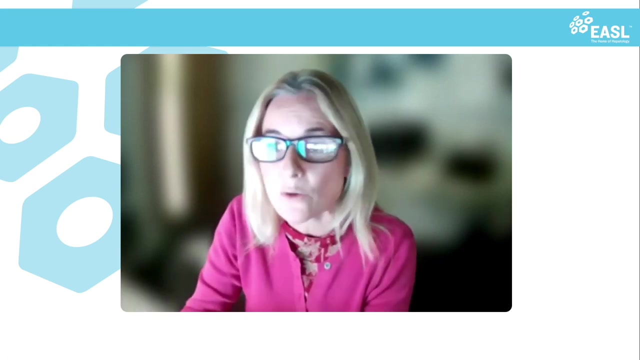 will be, you know, in the severely damaged environment, but I guess you know so. so, taking it back to to, I know that we, you know we, we sort of there's a lot of single cell data out there and thinking about the kind of the mechanisms, the signaling, the closed cell contact, you know. 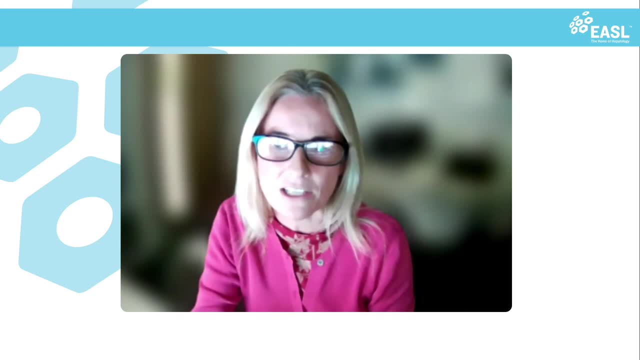 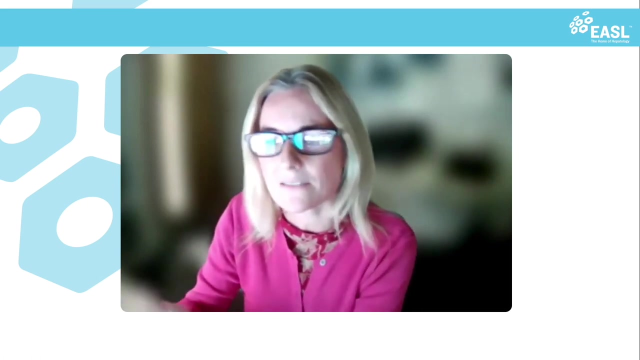 the computational methods that have come out of single cell biology I think will really improve our understanding of, you know, cell connectivity and the pathways and the ligands that are responsible for neighboring cell signaling. now maybe you know, in that context of that severe liver tipping point of, of this liver so so badly damaged, we might be able to understand how we can. 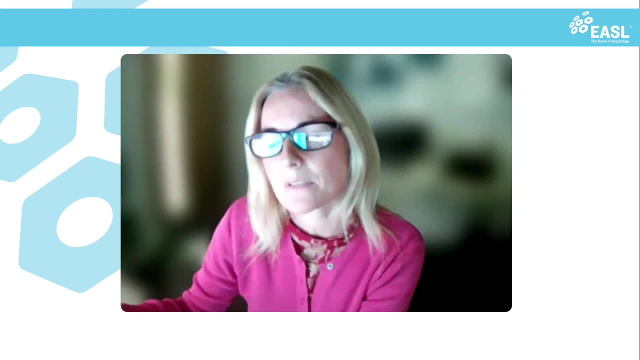 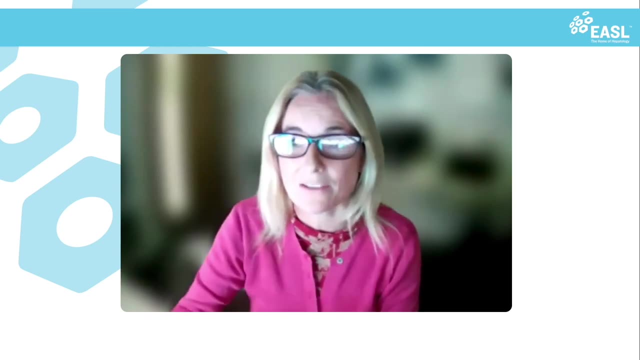 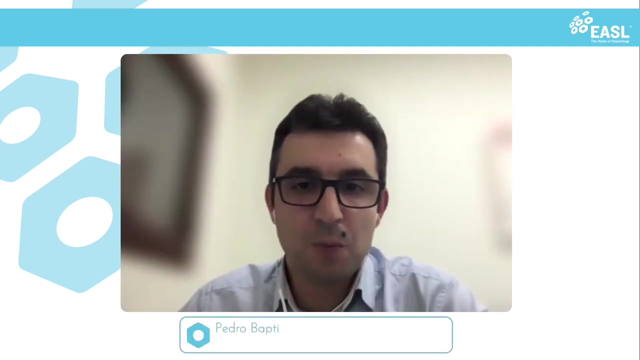 improve those impaired mechanisms by looking at these kind of computational methods of cell cell contact and link in with the sort of work that yourself, Frederick and Tobias are doing to to improve that. so yeah, you're somehow alluding to the situation where you have reached an irreversible state, right? 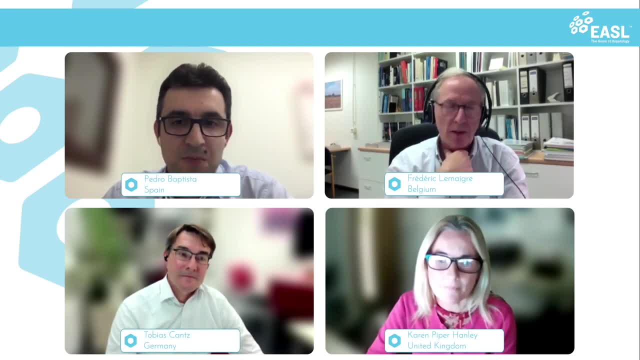 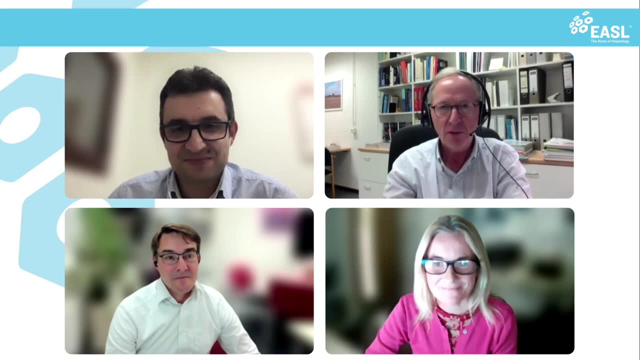 um, I, I'm what I'm. I trained as an MD, but I'm not a clinician, so I cannot tell you how the clinician can address that. but phenomena of irreversibility have been studied quite well by a number of developmental biologists, including some who teamed up with computational biologists, because when you define the cells, I mean 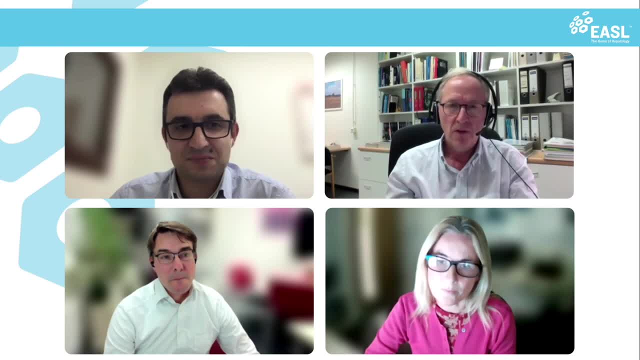 in terms of gene regulatory networks. these networks, you know, they evolve, they switch from to one state to the other, uh, for instance, during differentiation, or during day differentiation, or when they move to a deceased state. but you can computationally really measure when you have reached the state of. irreversibility of yes or no. so you can try to do this by using your own standards as well, but if you can't do it right, then you have to try ideas something like this: you know, and, as a result, you're basically even more likely to be in a state of irreversibility than you are in a state of irreversibility or yes or no. 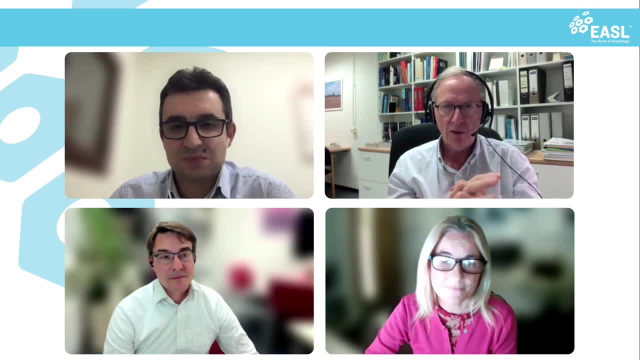 no, can maybe define this stage of irreversibility at a clinical level with a patient, but i'm quite sure that in the future, by looking at profiles of gene expression and strong computational methods, we will be able to define whether we have or have not yet reached such stage of irreversibility. 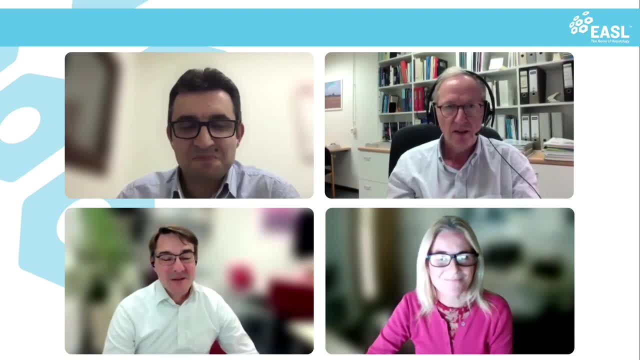 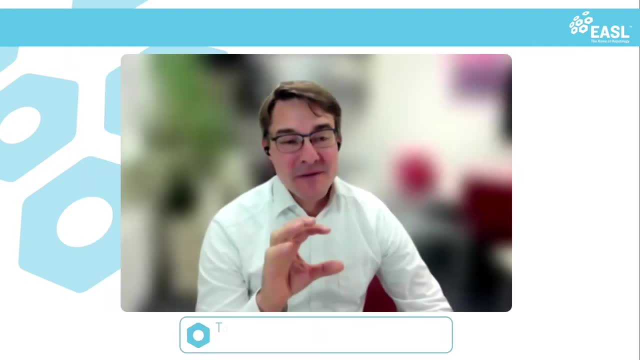 yeah, yeah, but maybe i i can step in here so i fully agree to you, but i, i still want to wish, let's say that if we, if we interfere, maybe this, this one cellular compartment, and change this a little bit, which might not be irreversibly damaged, so be it. maybe cell itself, so be it. 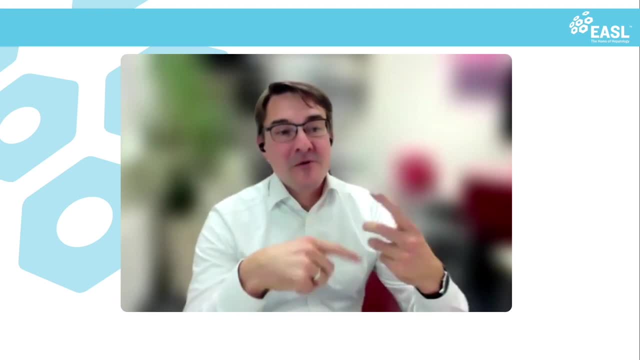 sinusoidal endothelial cells and we kind of reprogram those to a, to a state that these might then influence other neighboring cells that might also slightly switch. i think what we have learned from from all these developmental studies, but also the stem cell differentiation or stem cell transplantation, 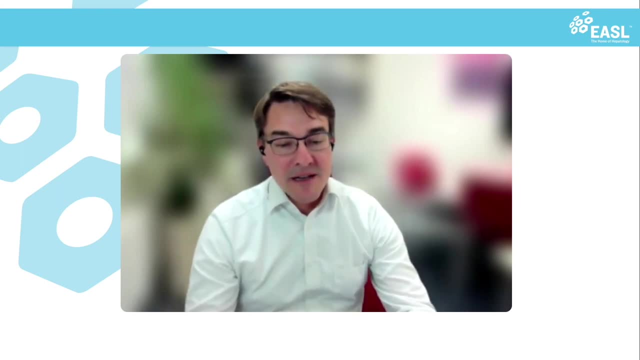 studies is that that we have a distinct phenotype in our in vitro dish, but this might change in vivo, depending on the environment, rapidly, very fast and also, let's say, timely in the suspect, during then being exposed to the stimuli of the neighborhood, and i i'm far away from understanding. 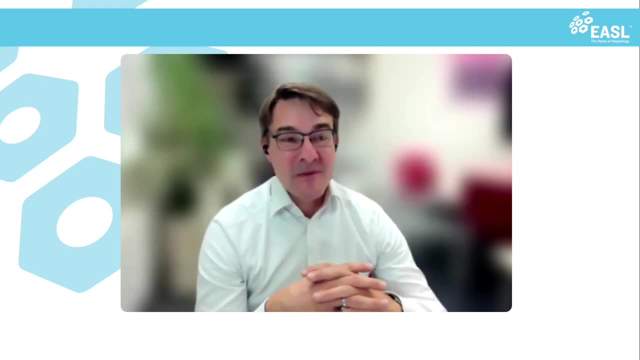 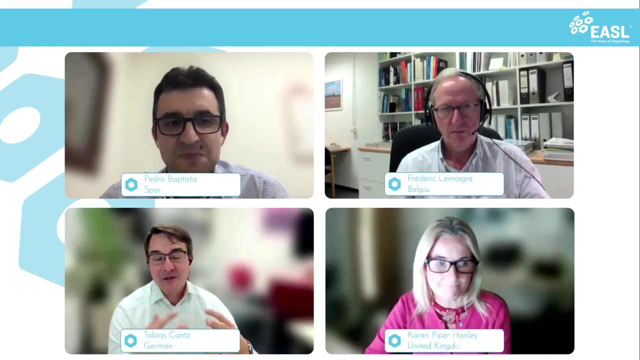 how this might happen, but i still want to wish that we might have to like it like a stepwise um. now then, to come back to art: stereotypical хотел for rates and今天 researches. plus if the use talked at the same time to. 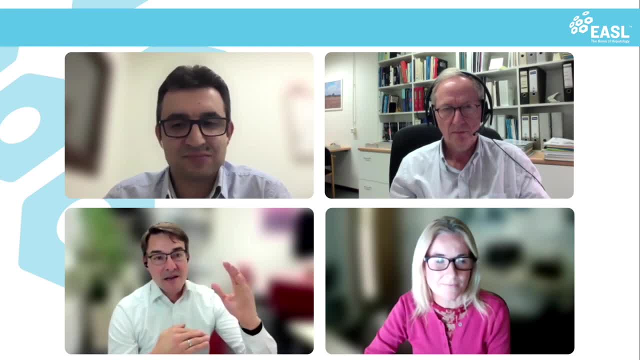 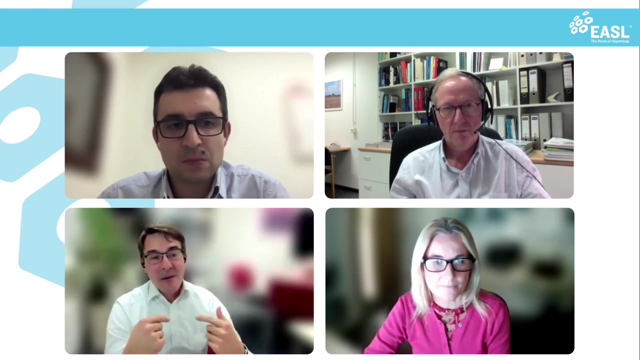 more. see that there, that that you see this, that will seem then not be able to export something into the biliary tree because it's it's so just blocked. but, as i mentioned, if you can step by, we stepwise regresses a bit. maybe then hepatocellular function also can. 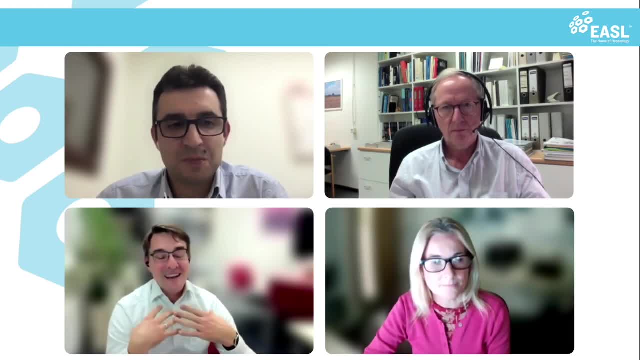 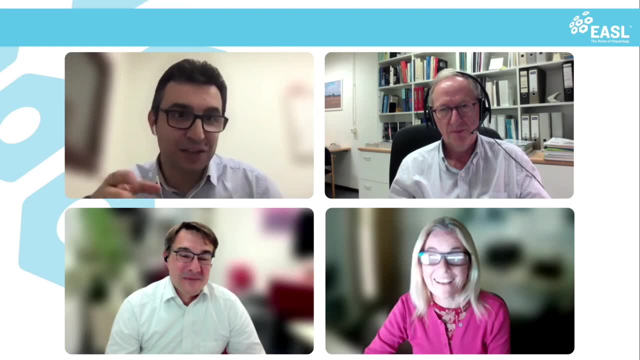 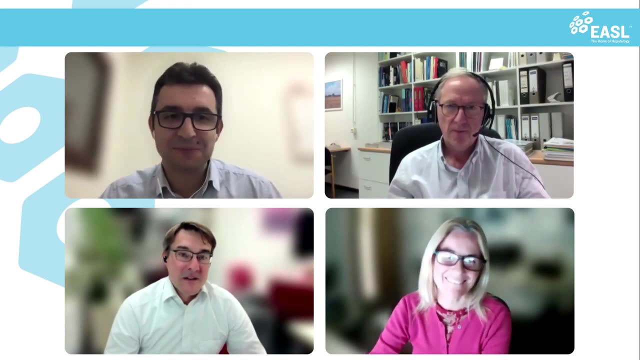 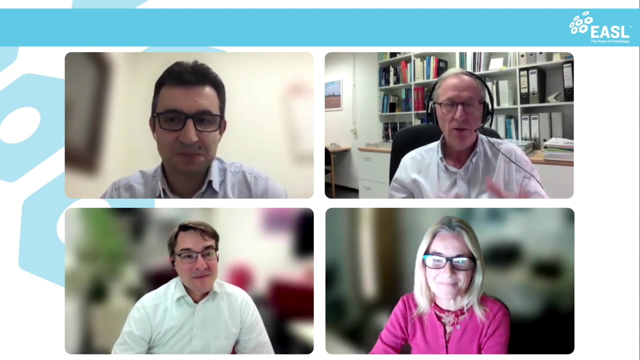 be plastic and and can we resolve? so at least i want to wish this- maybe stepwise cell therapies, taking that into consider, and those mechanisms, yeah, modulators of, yeah, with small molecules, regeneration, regeneration, whatever, yeah, at the same time, you're giving a fantastic example- tobias, when you mention you need to have hepatocytes which have the, the appropriate. 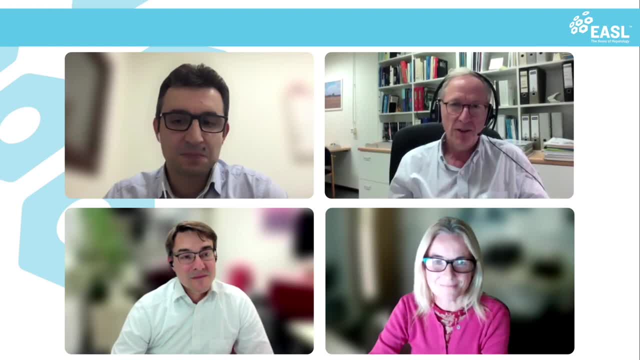 apico basal polarity. how do you get that? you need endothelial cells around so you want to regenerate hepatocytes. you are not going to succeed if you are not going to restore endothelial cells. you are not going to restore endothelial cells if you don't have a good blood flow and so 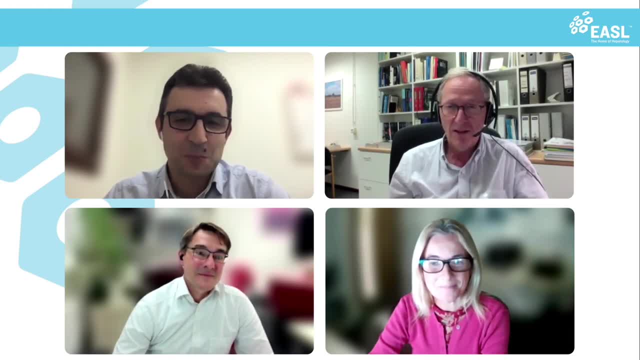 that's. this brings us back to the main difficulty. we still need a lot of information on how all cells- not just one cell type, not just the main cell type, but all cell type- how do they coordinately develop this? these are one of the major limitations of most of the work in. 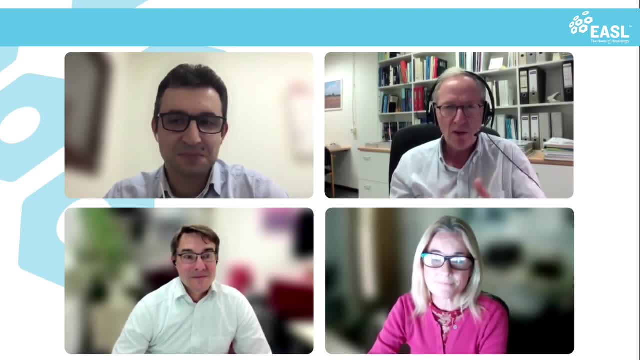 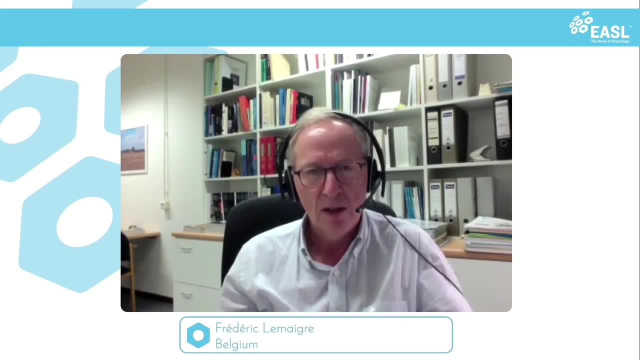 developmental biology, we have been looking at most of the time at one cell type at the same time. now single cell technology is progressively bringing more information about the coordinated cell types. the difficulty is that people are slightly overwhelmed with the amount of data and that they have to be able to extract what is critically important for being trump to allow. 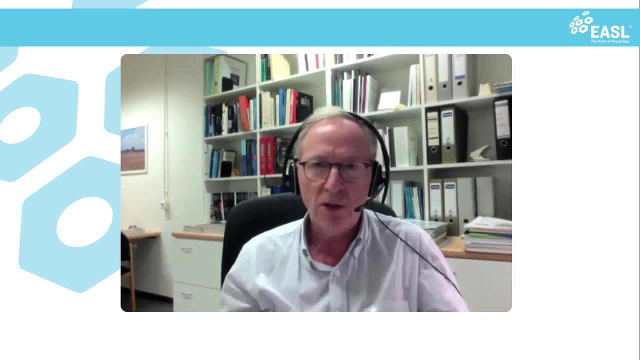 people to transpose it into a therapeutic strategy or even into a bioengineering strategy. so that's the limitation, one of the limitations today: too many data is good, but too many is hard to interpret. so i would just like to close before before we close, to just ask one of the questions we have in. 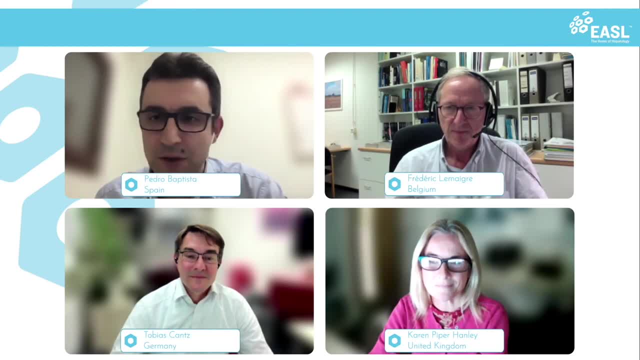 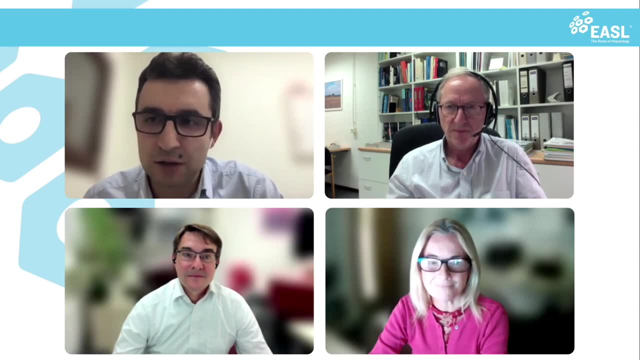 the chat and i'll just ask you one of the questions we have in the chat and i'll just ask: ask it generally, so whoever wants to to answer it go, please go ahead. so we talk about inflammation of the liver. is this both good and bad for the liver, as the organ is constantly under insult? 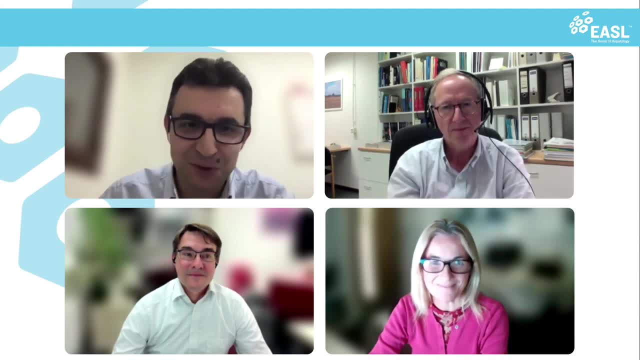 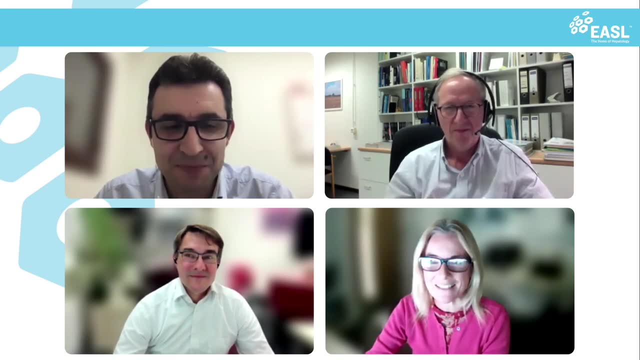 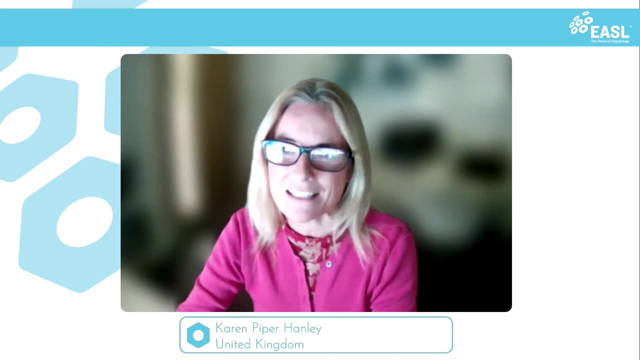 and may be required for function. oh, good question. so who wants to go ahead and and provide an answer to this? well, i, i think it. you know, it is both good and bad. you know, i think there have been attempts at, um, you know, for example, i think, was it the tgf beta inhibitors that? 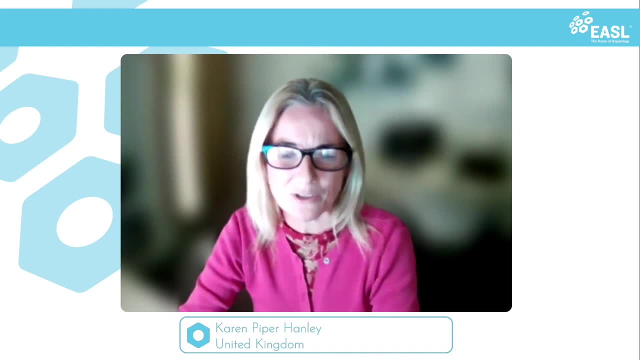 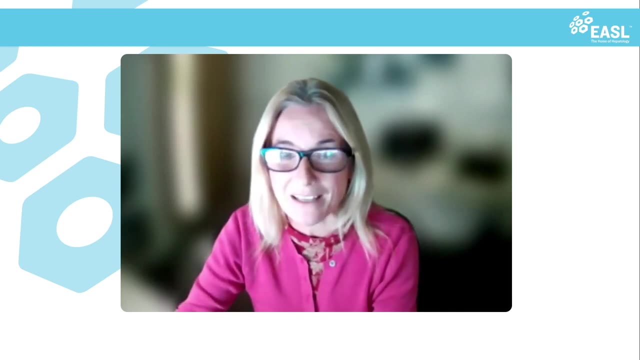 many, many years ago, uh, people tried to use to improve liver fibrosis and they actually made it worse. so that suggests that you know from from an understanding, the, the kind of inflammatory insult and and actually so it turns out that inflammation is both good and bad. you need it for correct. 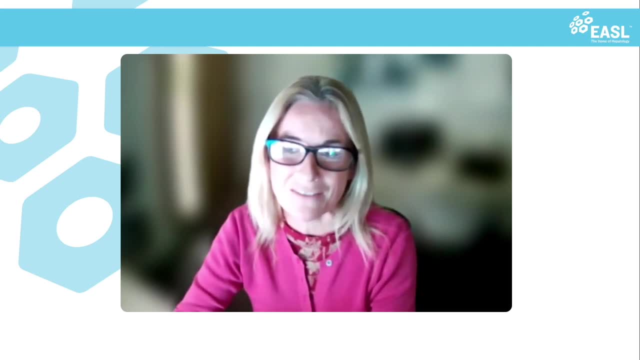 regeneration, correct um function of the liver, but clearly it's also there to, you know, to get rid of the bad stuff as well. so so it's, it's, it's a, it's a, it's a very important thing and and i i did some, So you can't just ablate inflammation and get a fully repaired liver, sadly. 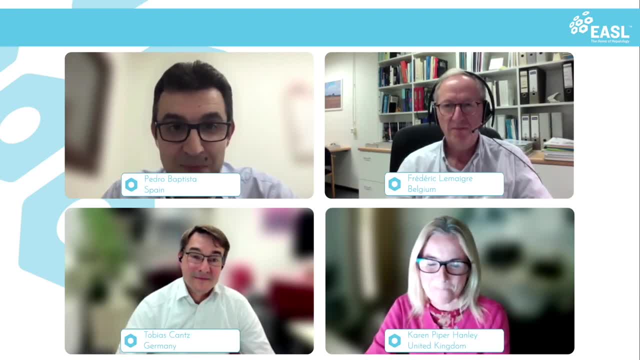 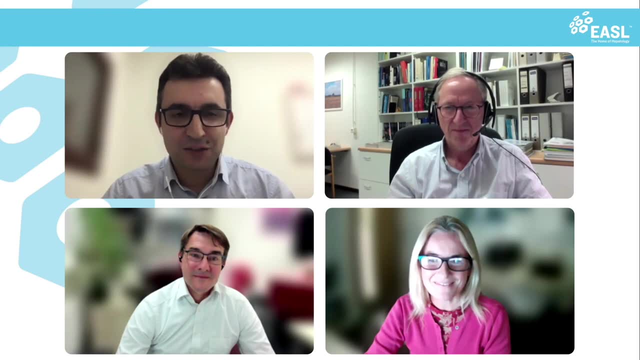 Thank you, Totally agree. So our time is up. I want to finish by thanking our three experts and three good friends, And I hope you enjoyed this. And just as a corollary of this, so if your liver is just gone, so wait a few more years.